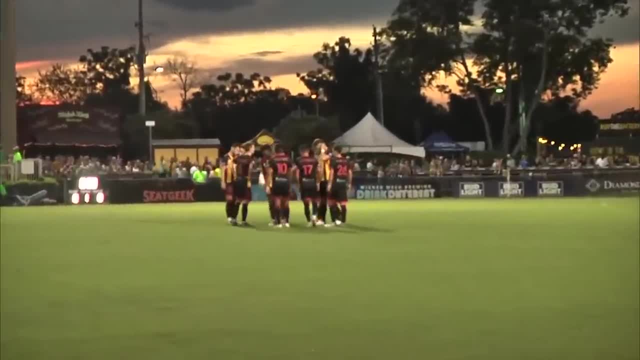 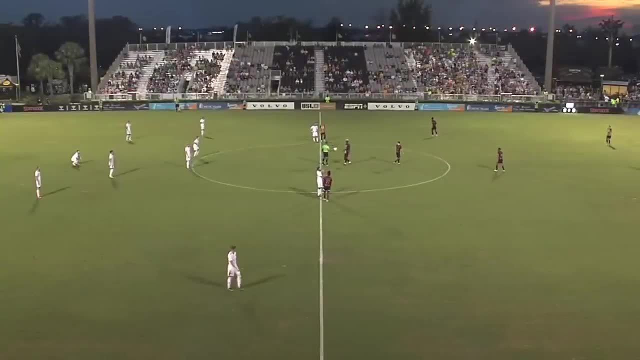 Let's just jump into the game analysis video. As you can see, beautiful, beautiful night at Patriot's Point. It's like 80 degrees or so, Humidity levels high but no direct sun 8 o'clock at night. Really really nice to start the game. 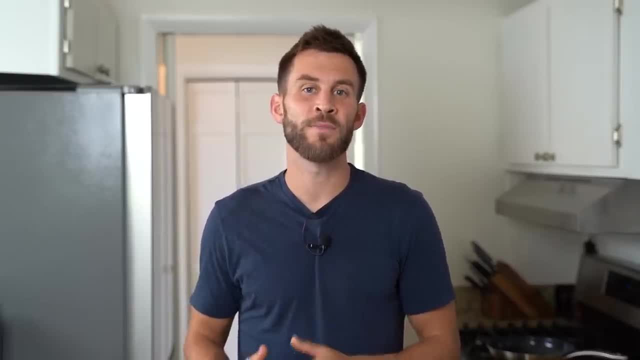 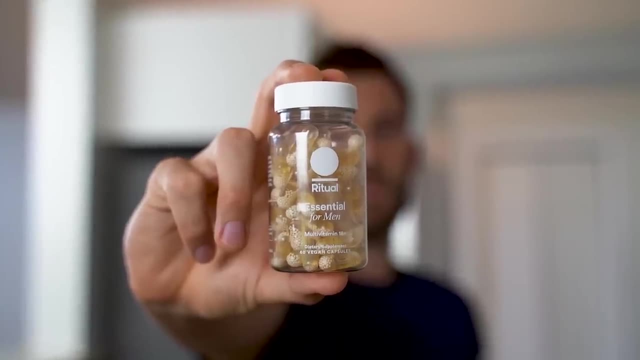 So before we hop into this game analysis, I just want to take a quick second to thank the sponsor of today's video, Ritual. Do you have a perfect diet day in and day out? Yeah me neither. Ritual helps people fill the gaps in their diet with no shady additives, colorants or fillers, Just two. 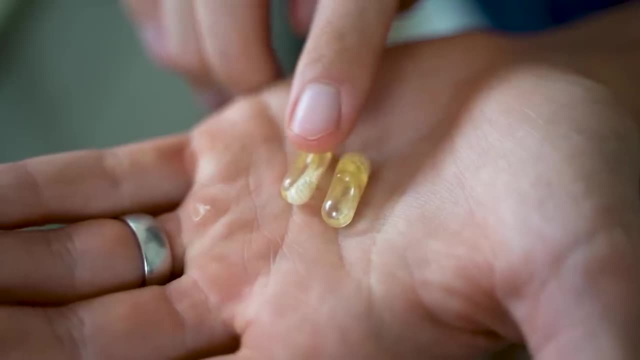 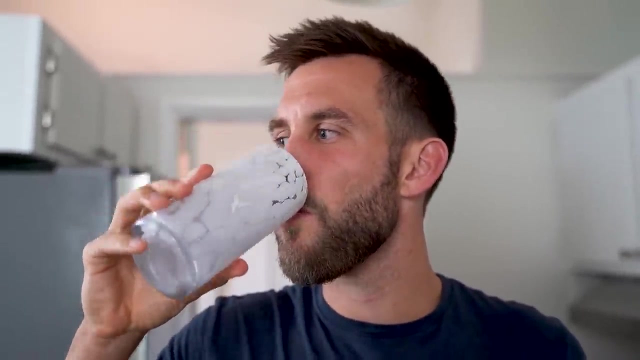 of these easy-to-take capsules provide 10 key nutrients to support a strong foundation for your health. I take Ritual because, as a professional footballer, I want to do everything I can off the field so that I'm reaching my maximum potential on the field, And Ritual is a brand that I can. 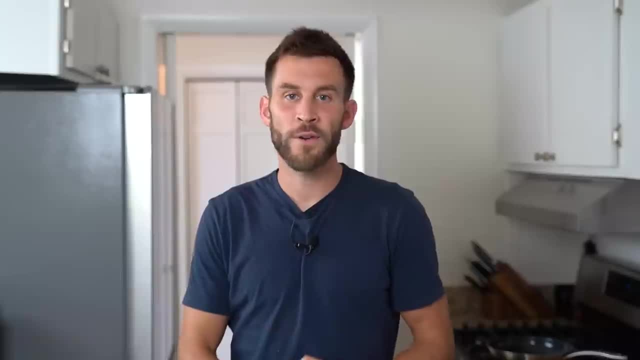 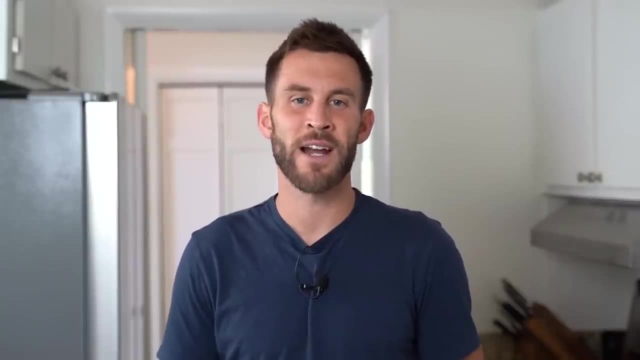 trust because of their absolute, complete transparency for all of their ingredients, why they use them and where they source them from. Ritual is the obsessively researched and transparently made multivitamin, And the Essential for Men contains 10 high-quality nutrients like 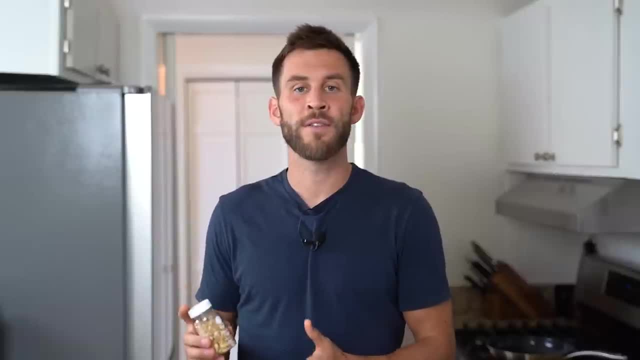 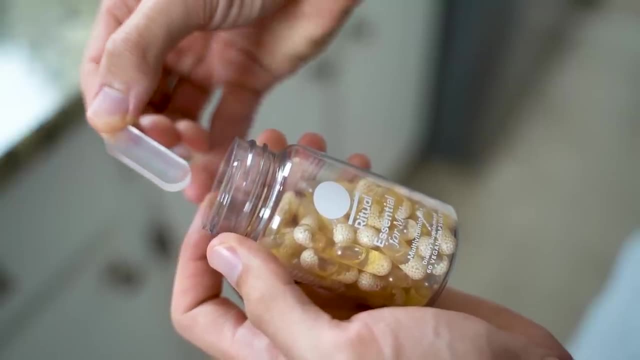 vitamin A, D, omega-3, and zinc. that are all difficult for men to get through their diet alone. The delayed-release capsule design is gentle on an empty stomach And there's a mint tab in every bottle to help keep your multivitamin smelling fresh. 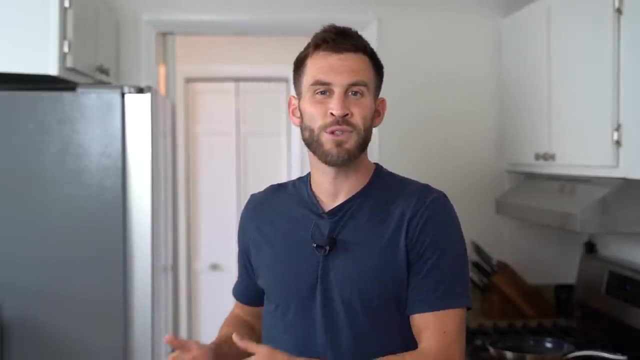 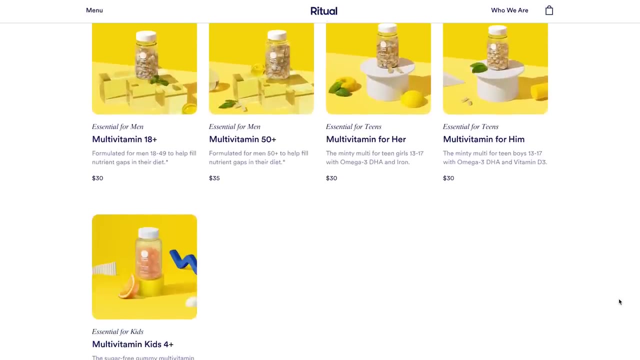 And Ritual has vitamins to support everyone. The Essential for Men is a multivitamin designed for men, but they also offer a multivitamin for women, a 50+, a postnatal, prenatal and even a teen vitamin Plus. they are vegan-friendly, non-GMO, gluten-free, allergen-free and contain no added. 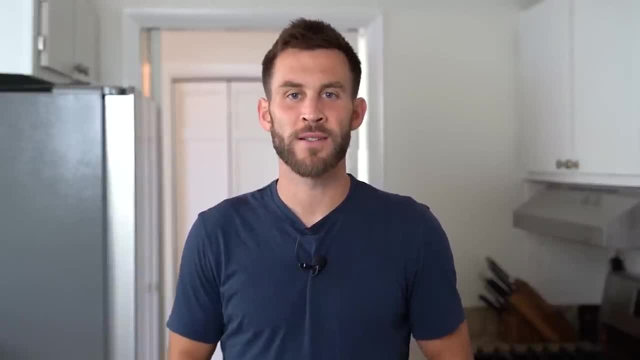 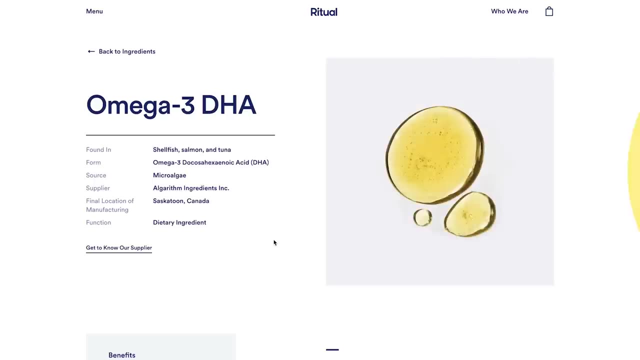 sugar. Transparency is at the core of everything that Ritual does, from the way the nutrients are sourced to the environmental impact of the materials used to ship thousands of orders. Ritual has searched the globe for the best suppliers and is completely transparent about where they source all of their nutrients, And Ritual has a wide range of nutrients. 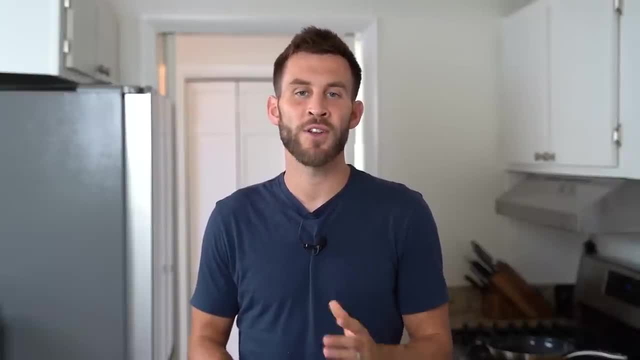 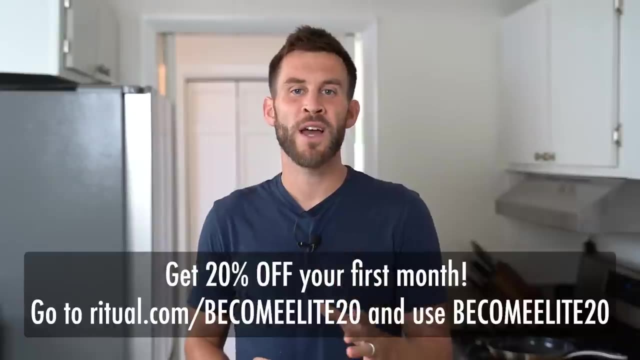 all of their ingredients. It's only a dollar a day to have 10 high-quality nutrients that your body needs delivered straight to your door every single month. no strings attached, no extra charges. Ritual are offering 20% off your first month. by going to ritualcom, slash, become elite. 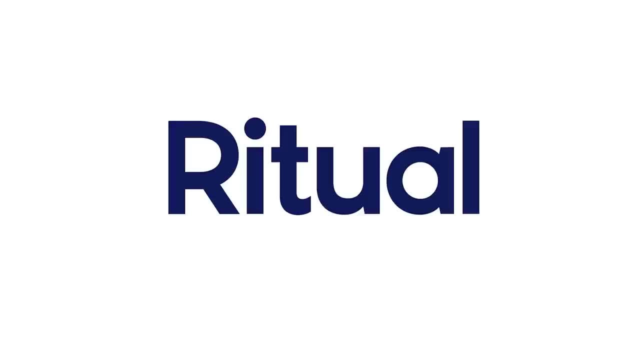 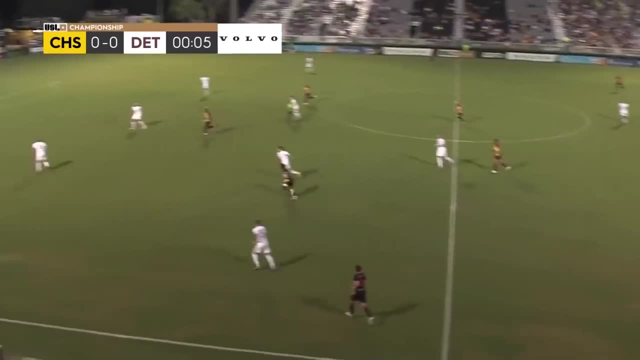 and using code BECOMEELITE at checkout. Thank you once again to Ritual for sponsoring this video. So, anyway, we're going to start with ball. We're going to be the black, yellow and a little bit of red team with the ball, And Detroit City is going to be in white. So we start off with a kick. 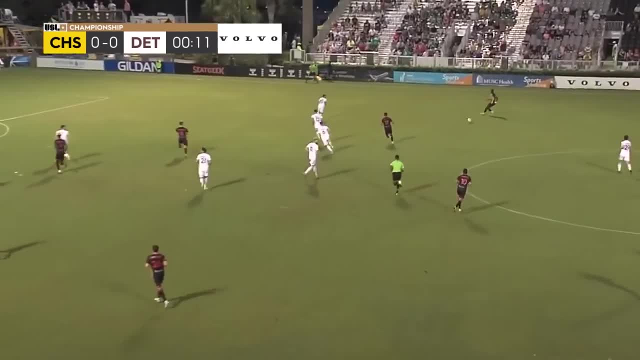 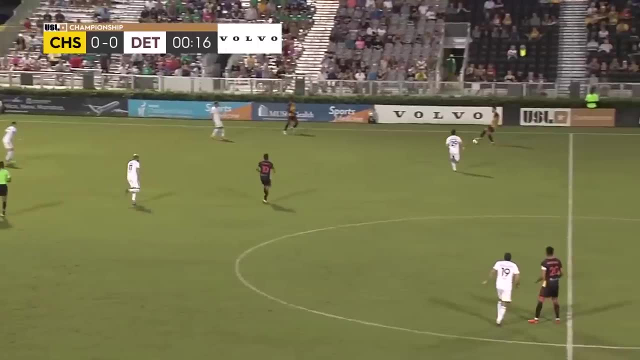 and opt to go long. We fail to win that first header, but bring it all the way back and switch over to that far side. DZ- my wingback- has the ball, decides nothing's going forward. He's going to play it back to me. Same thing as DZ, kind of. 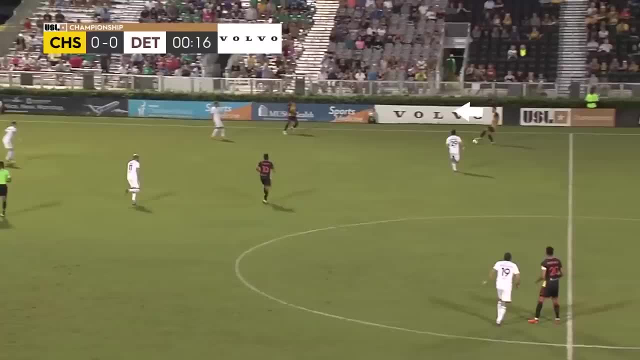 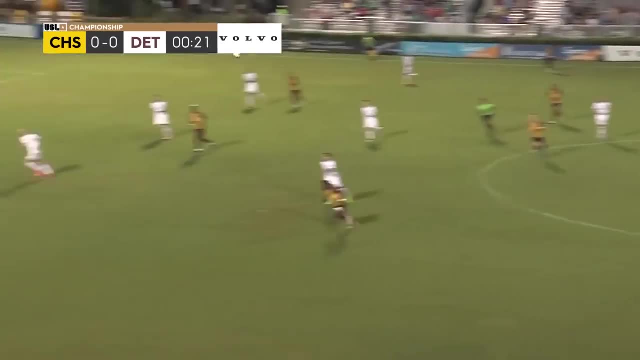 thought there, I'm not seeing much down this right side. I could maybe play into Romario Piggott. but then, first couple seconds of the game, let's establish possession, Let's swing the ball side to side a few times So I play it back to my center. center back there. Here's my 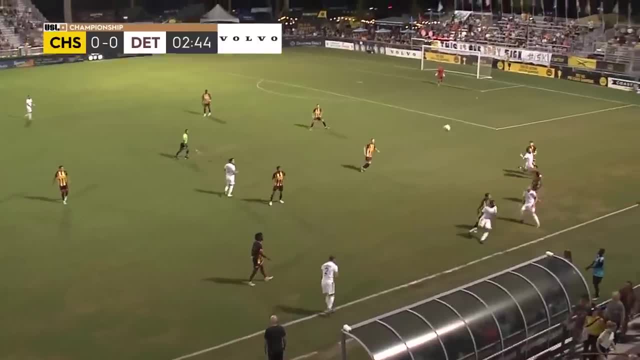 next touch in the game, Detroit City FC is going to have a throw-in. They're going to throw it all the way over to their top striker. We're already pretty out of position. This is our center center back. This is our left center back. I think I'm in a good position. 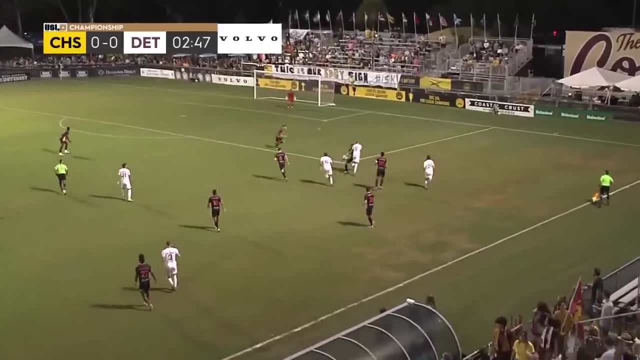 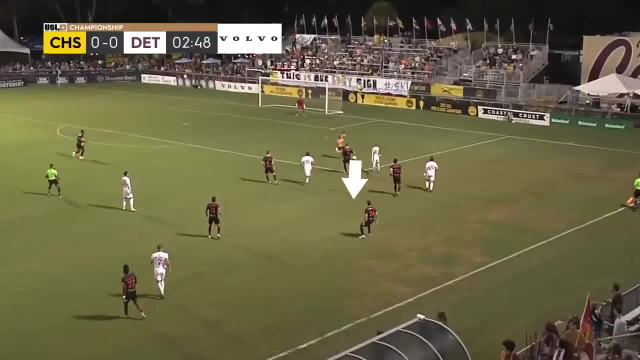 where I'm centrally kind of covering, but I still can get over here and win this ball. And then with this I don't want to clear it forward into this mess of people and get a deflection And the ball is going to go in behind me and maybe lead to a goal. So I'm just going to chip the ball out of. 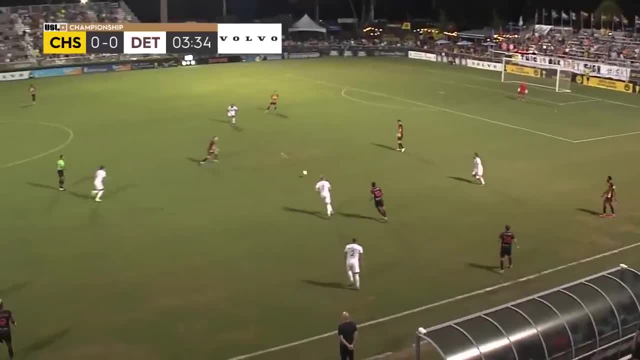 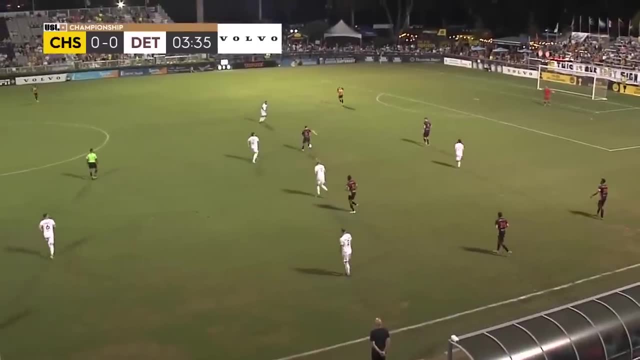 bounce easily, safe and let everybody get back into position here Now, as this ball comes into my center mid, I'm going to drop like 10 steps quickly to create a good passing angle. So Robbie can just play me back the ball I can. 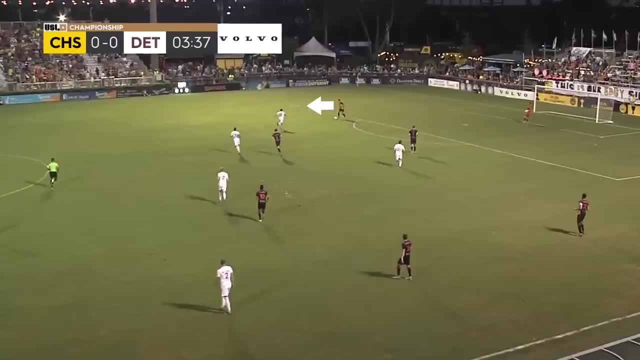 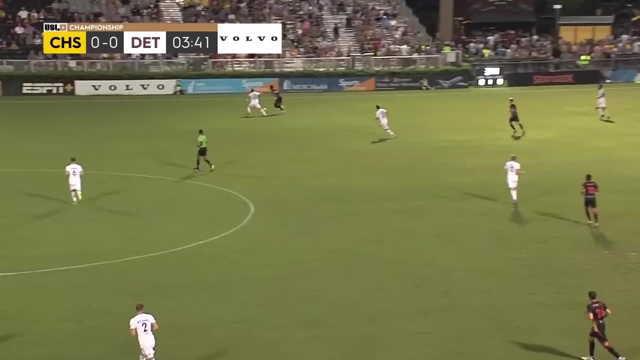 I have a little bit of time on the ball, face forward, open up my body and find DZ, my checking wing, back coming down the line. I can find his feet there. He has a good turn and then starts to drive up. He ends up getting fouled here. Here's the free kick right here, But basically. 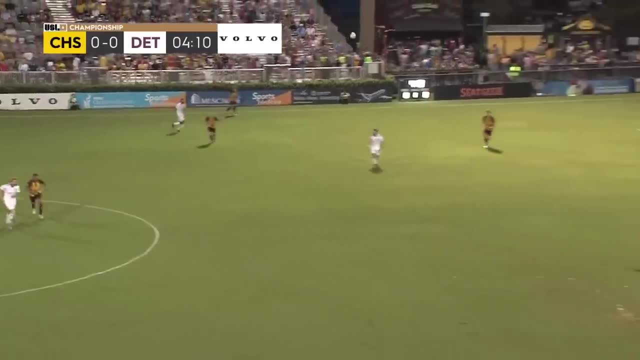 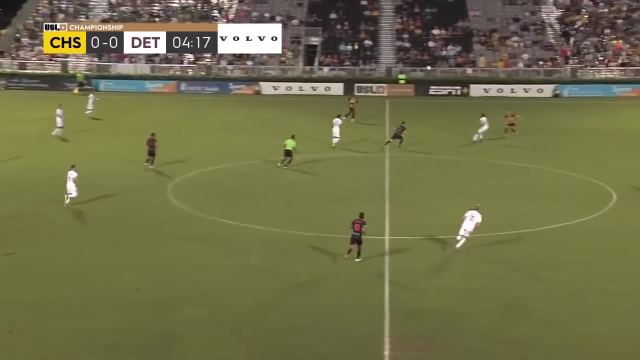 I start to look to go close into Robbie, I kind of decide it's a little bit too tight here. I'm just going to switch it over to AJ, my left center back, and then we can build up on. that side Ends up coming all the way down right back to us. 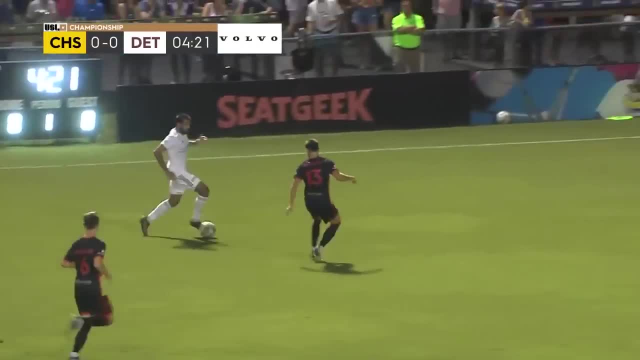 over my head And now it's just 1v1 defending on Botello-Foz Here. all I'm thinking is delay as much as possible and keep him wide. That's what's going through my head right now. I don't. 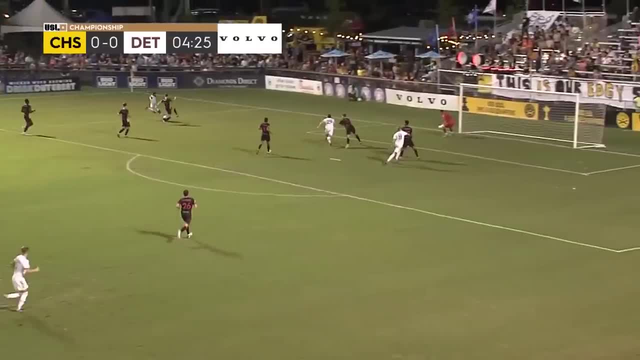 need to dive in. He's got really good control of the ball right now, So I'm just going to keep him wide, keep him wide, keep him wide, And as he winds up to cross the ball, I'm lifting up a leg. 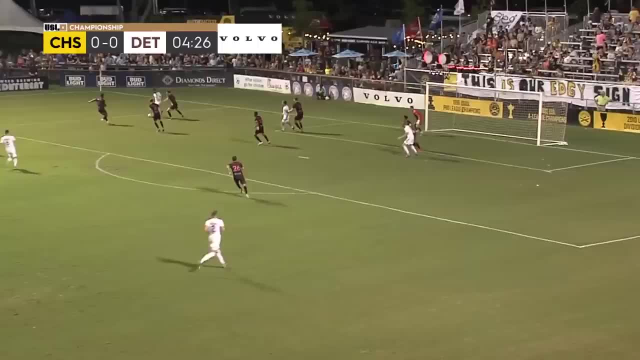 to block that. But still, as you can see, I'm still able to cut if he decides to chop that ball back faking that cross. And again, I'm keeping him wide. I'm in a good position, We have our guys. 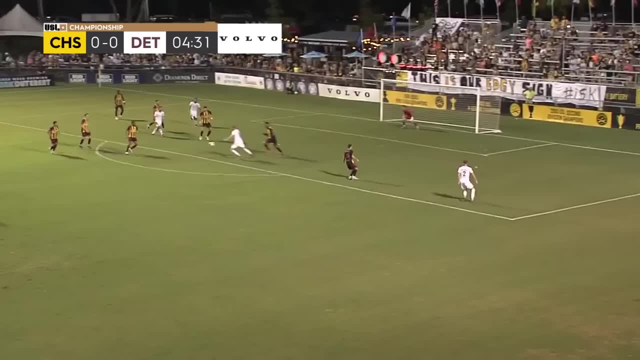 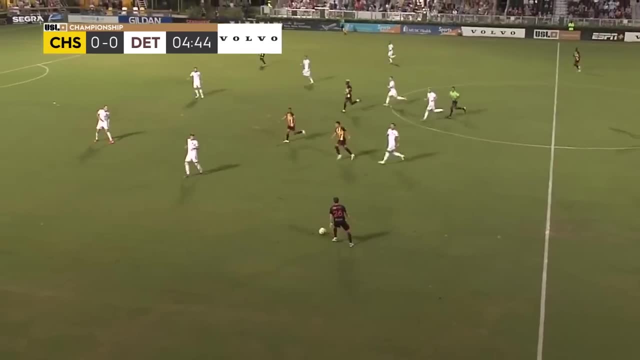 back now. I think that's a really good defensive action, Even if I don't win the tackle there- And, as you can see, we end up winning the possession of the ball, And that's a great team defense right there to stop Detroit City FC's attack. Now ball back. 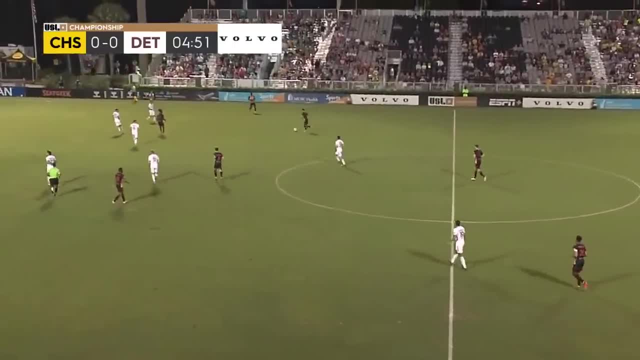 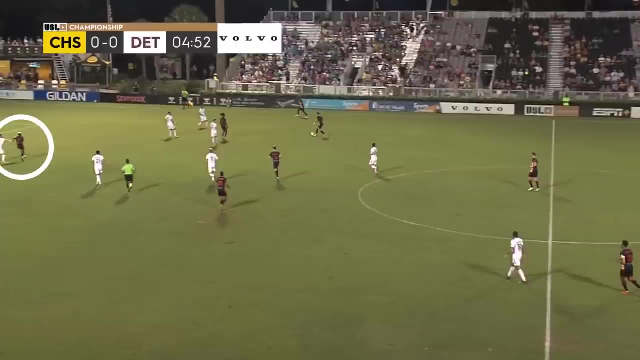 into Robbie. He has tons of time to switch it over to my side. A little bit rough of a first touch, but just driving forward into the space. And then I see this high line here and I see Augie running towards the end line, So I'm just going to try to play him in behind. I should have played a little. 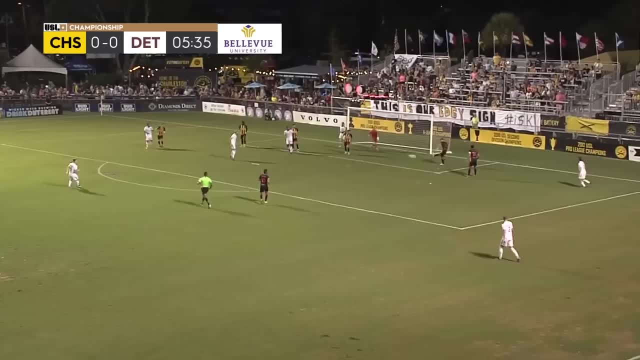 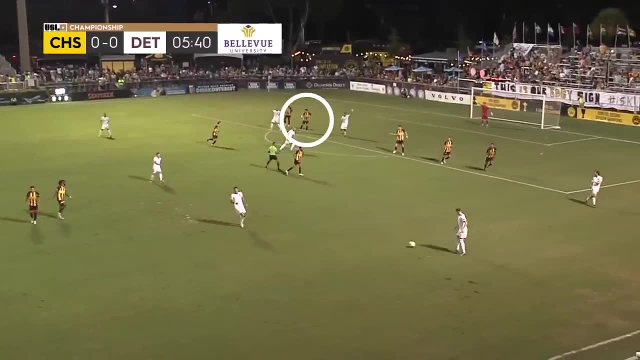 bit softer, a little bit more wide, so we could have got there. But I think that's a good decision With the right pass. just the execution needs to be better there. Detroit City FC wins possession of the ball. now I'm checking over my shoulder trying to organize back here. I see three white 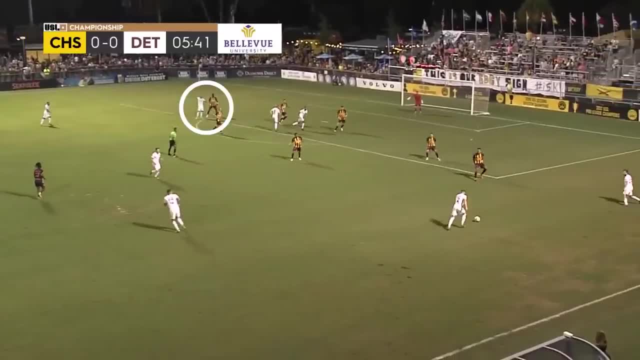 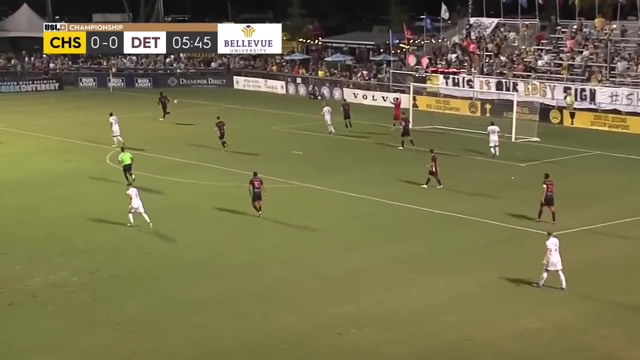 shirts around me, So all I'm doing is just trying to pick up the right runners. DZ's got his guy. I'm yelling to Pat, you know man coming right shoulder, right shoulder, so he can pick up his guy And then I can be on my guy Again. I don't end up making an action on the ball. I kind of. 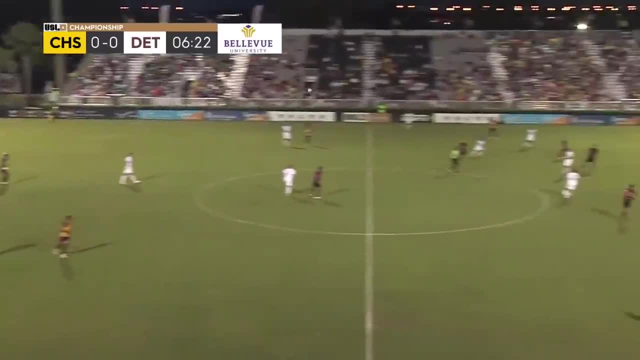 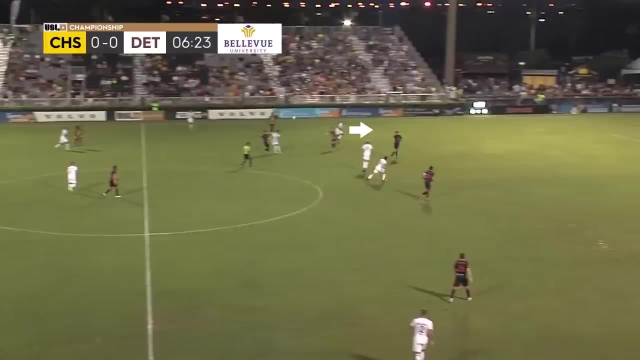 just let the ball go over my head, But just the organization of the center back there. I think to block all those runs is really important. Ball comes into me. I try to chest this ball down because Botelho-Faz is making a run behind. I know I have a little bit of time, That touch is a little. 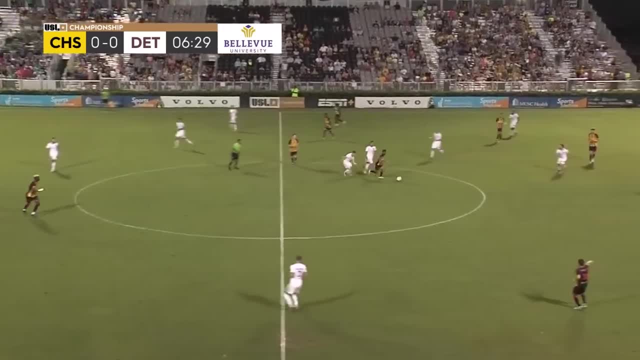 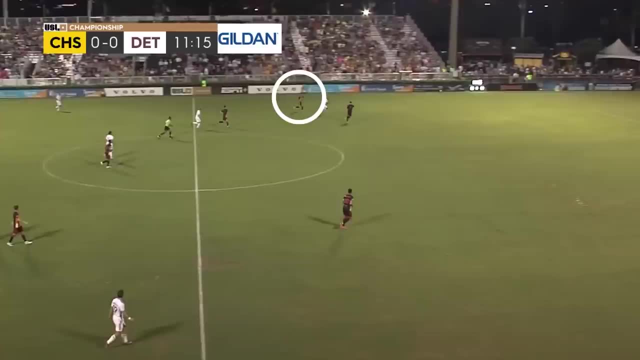 bit heavy but still end up maintaining possession of the ball here by chesting that down, Just going to be a little bit cleaner there, but I think that's the right decision there as well. Then ball over my head. I think I can win this header. I think I can head this behind me. My worry was: 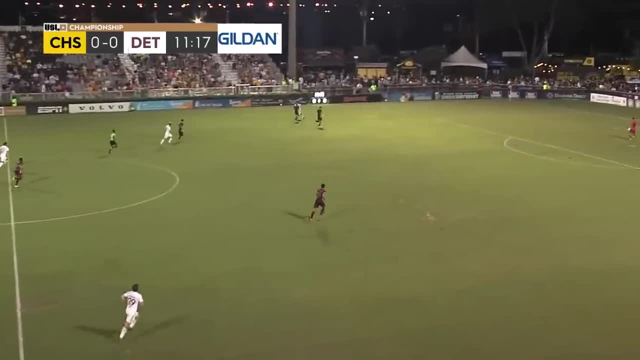 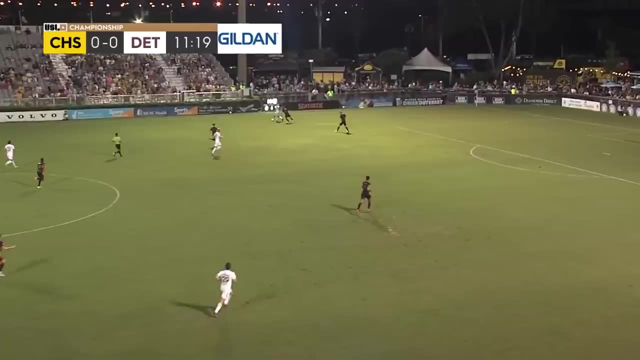 that I was going to have a glancing header and the ball was going to go in behind or something. So I just let that ball drop and decided I'll just stand him up, force Botelho-Faz backwards and wide and allow team to get back. But looking back at this, 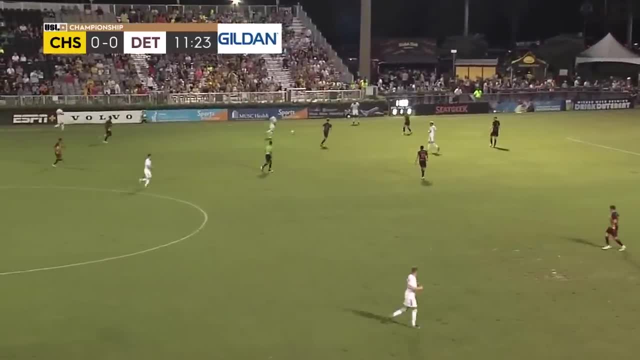 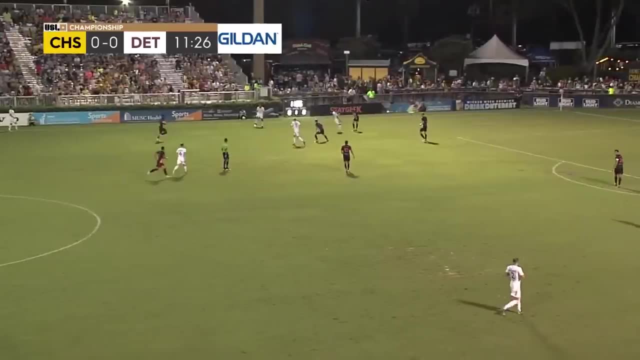 and I even think immediately after this play I was like, yeah, I should have just won that header here. But again, I mean, you know, we're just being safe conservative. They have the ball on the side of the field allowing our team to get back. I'm just picking. 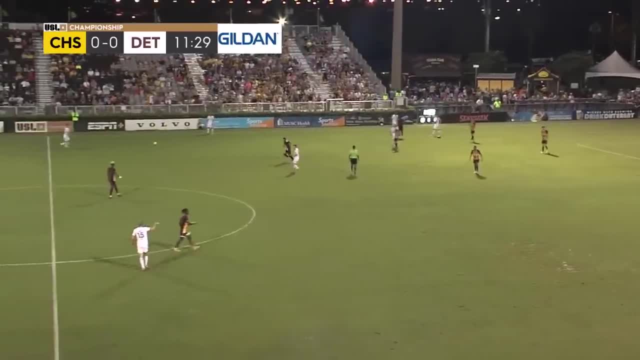 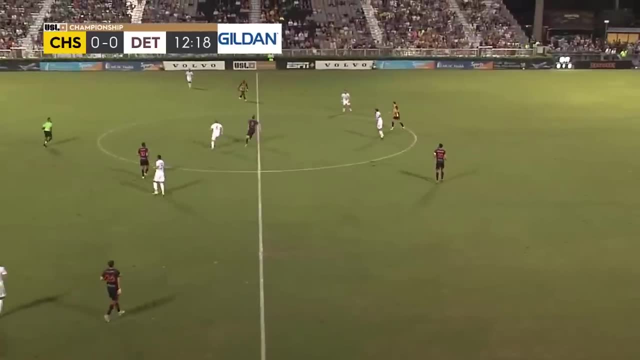 up the deepest man and just waiting for my wing back to get back. They play it all the way back And you know, even if there could have been a better action, still there's nothing dangerous coming from that play. Ball comes into the center, center back Pat, he steps up. 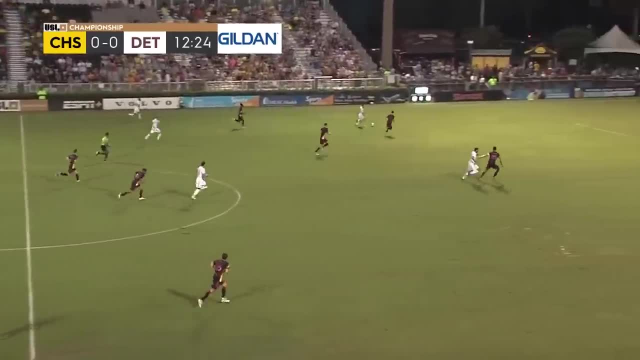 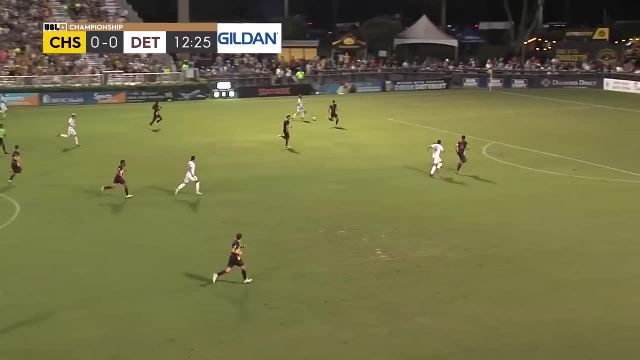 Kind of bobbles the ball. So it leads to a little bit of a counter and very, very similar situation again: keeping them wide, delaying as much as possible So Pat can get back in position because right now we're 2v2.. So just delaying, delaying, standing, hoping no upright here. 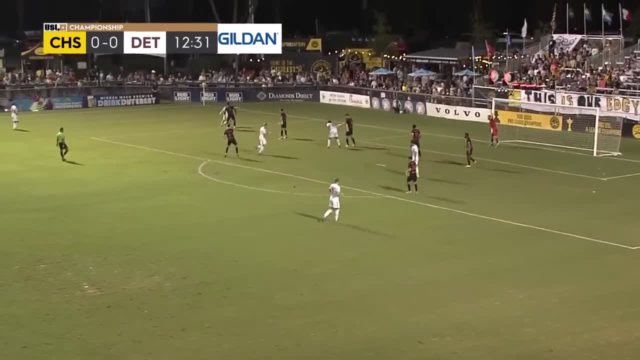 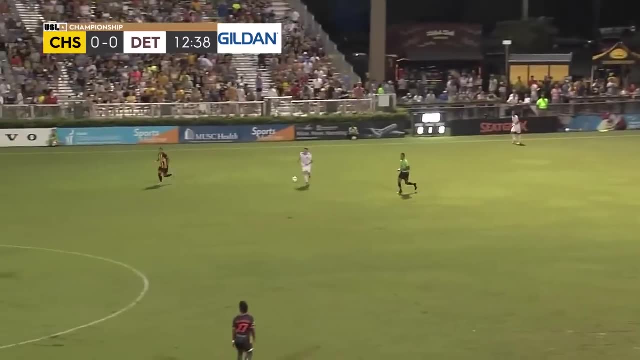 And he ends up crossing the ball right into Pat's head because Pat was given enough time to get back. Then DZ wins the ball over here. Great defensive action over here clears the ball up And although we don't get to the end of it here on the ball, I think again: very good team defense, good decision. 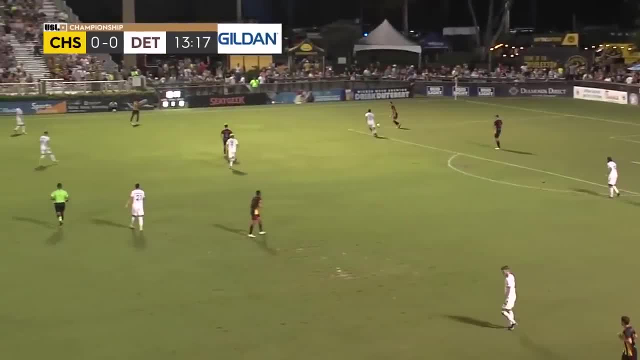 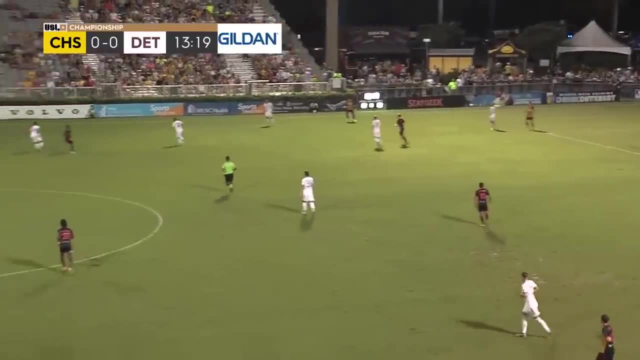 making over here Receiving the ball from my goalkeeper, Ugo, I'm taking a touch wide. I think I should just play DZ here quickly. I take a couple touches here trying to look for my striker Ends up deflecting. 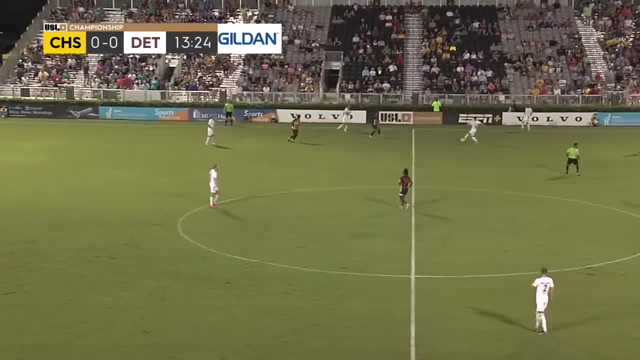 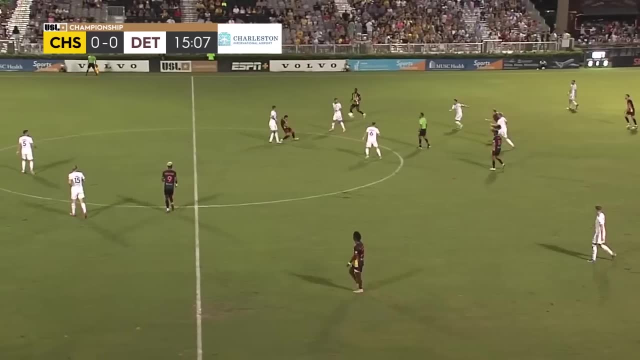 not what I want. Yeah, just took one too many touches there And I think I could play the simple pass to DZ my wing back, Just winning that header, popping it forward to Aiden Apodaca. He's unable to bring that ball down, But again, just kind of like clearing the ball out of the 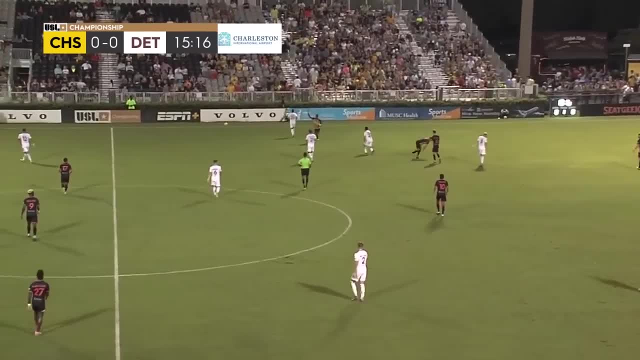 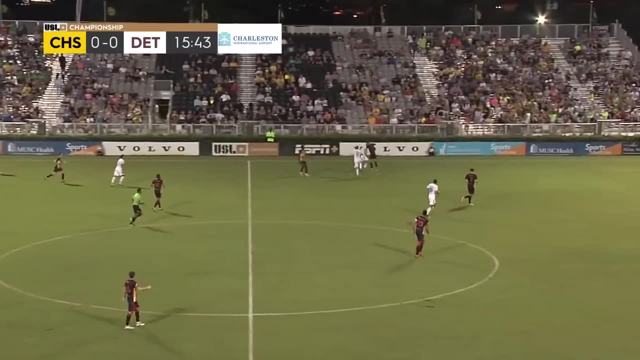 danger. It's kind of messy here, but just winning a couple headers And unfortunately ball goes out off of me. So now it's Detroit City FC's ball. Long ball from the goalkeeper, kind of just winning that header, getting big straight down into Romario Piggott. 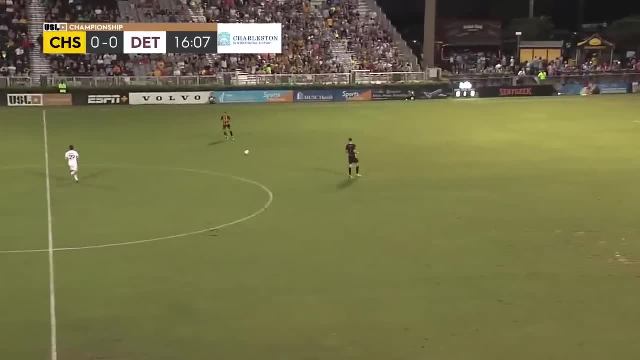 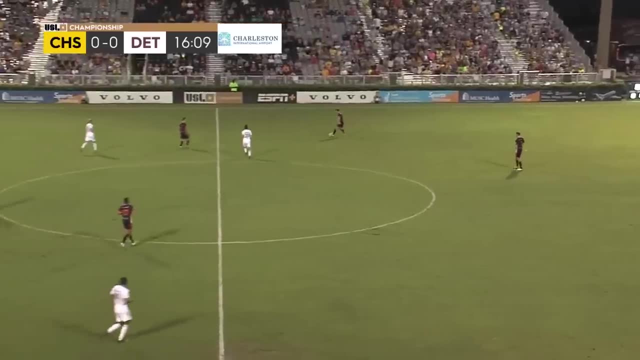 And now we can keep the ball, switch it over the opposite side and build an attack now. Now I'm just receiving the ball from my center center back. Pat Hogan Robbie, my central midfielder, is kind of popping into the space. He's got a guy about five yards away from him. 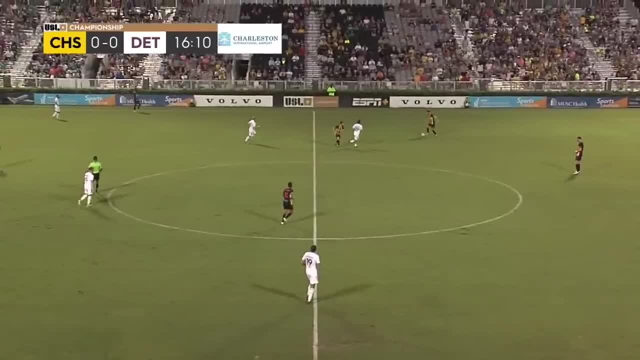 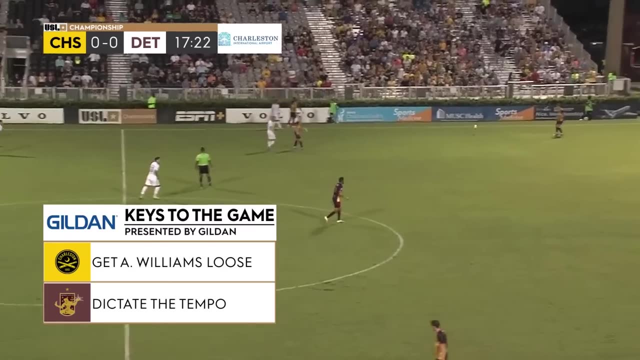 So I just pass him in the ball, say bounce right back, man on whatever, I'm going to receive this ball. And again on this right side I don't see much. So just play back to Pat And let's keep some possession here And let's try to. 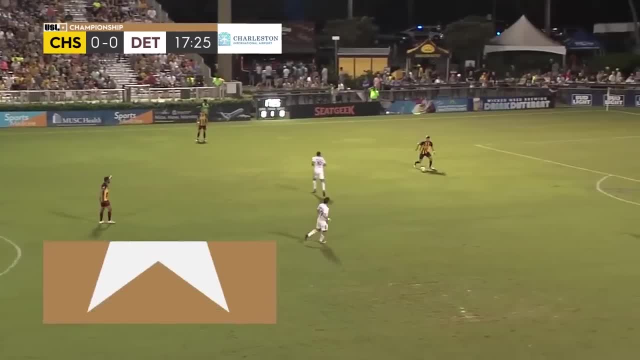 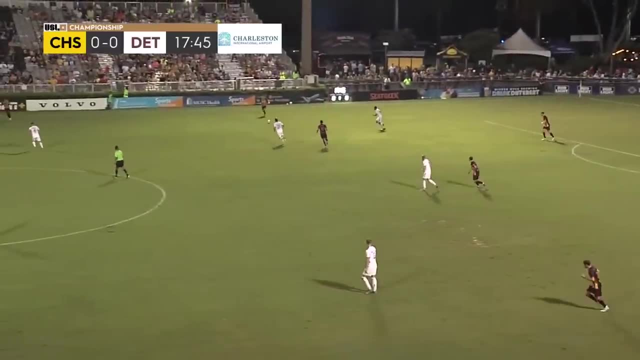 build an attack by switching over side to side, Receiving the ball from the throw in Once again, just playing back to Pat and swinging it all the way over to the left center. back, Ball comes into Roma who plays it out to me. I got tons of time and I got tons of space as well, And this guy's. 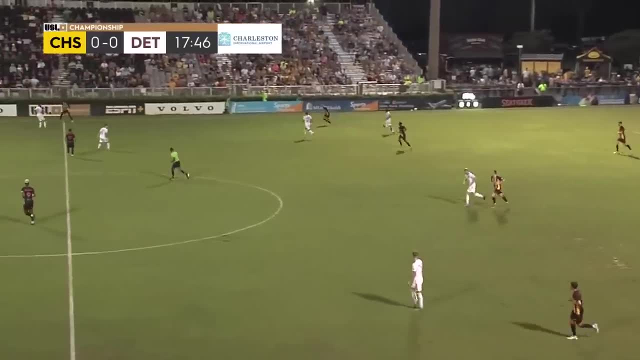 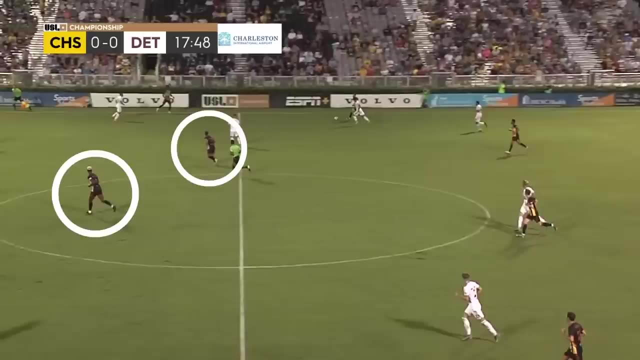 starting to make his pressured run, kind of rounding it. So I'm going to try to take that space and drive forward. But as I'm driving forward, I'm not seeing any passing lanes open up. These are our two strikers. Here's our wing back. I don't think it's on, So I'm going to cut the ball back. chop the ball with the. 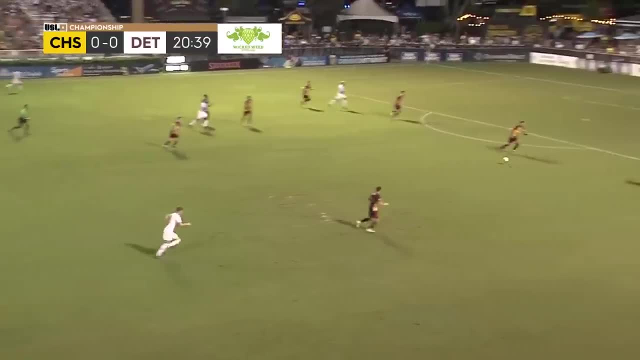 outside of my right foot. play it all the way back to Pat now And let's swing it over the opposite side Now. 1v1 defense from AJ. I'm just following my run. I'm yelling at my center, center, back that. 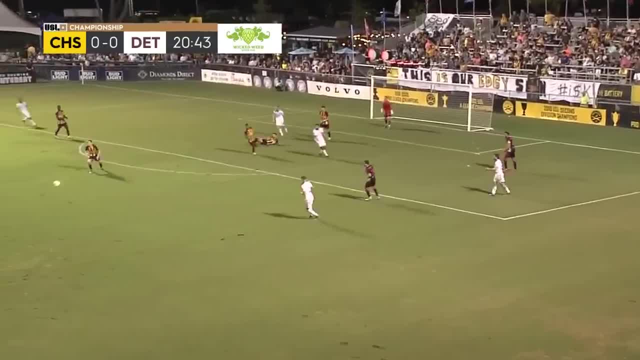 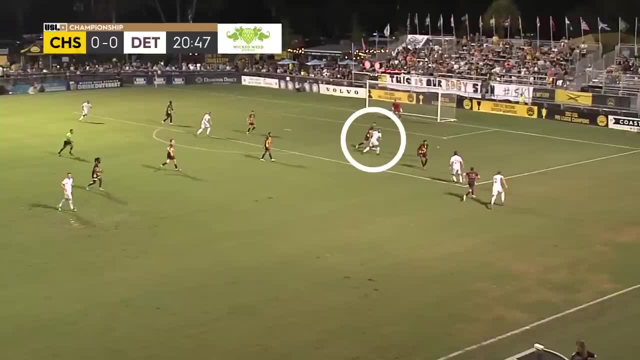 he's got a run coming And I'm just kind of being in a good area to block that that cross as it comes in. Getting back up Once again reorganizing, checking my shoulder, finding my man Pat's on his man, and just trying to track these runs as they come flying in. And so ball comes in. 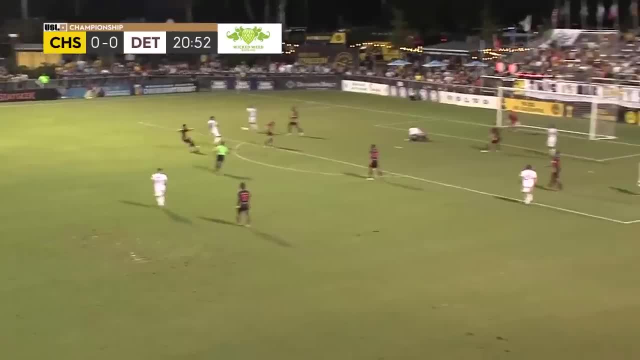 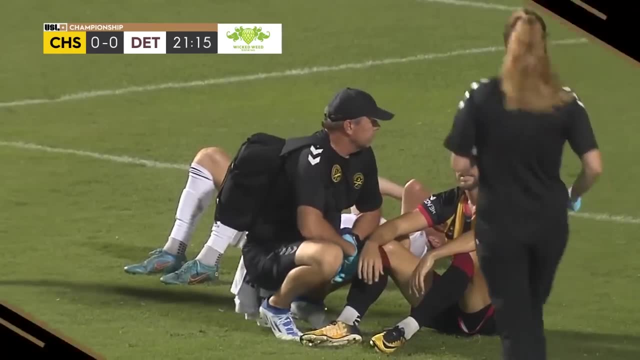 ball's crossed in, get up, win the header And then me and Roots just end up clashing heads here. His forehead comes in the back of my head. We're both okay, but just need to be checked out by the trainers And you know, this didn't feel too great, but no concussion symptoms from either of us. 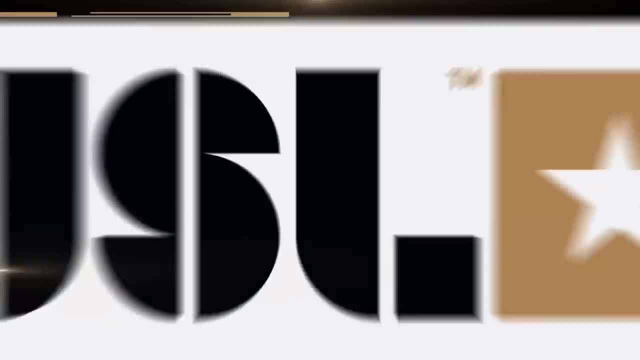 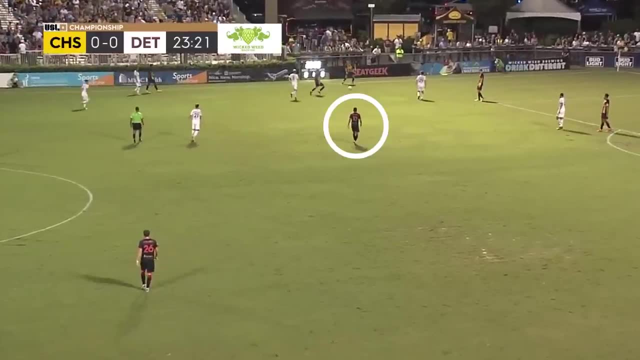 which is really good, But there's just winning the ball, little clash of the heads and both of us just drop Next play. I actually have the ball over here for the throw in. I'm going to throw it into my checking central midfielder here. I think Rome is on. I didn't see him at this time. I'm gonna be. 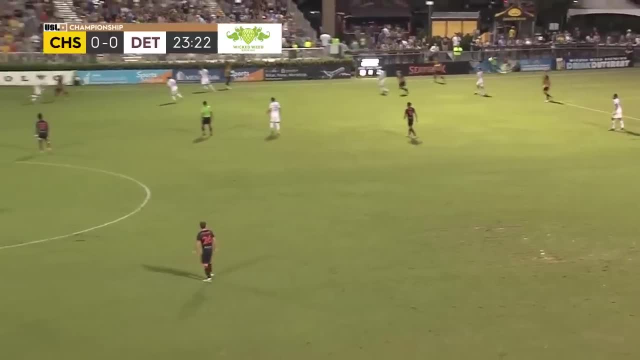 a hundred percent honest, Just focused around me, Ball comes back to me And then, with the left foot, I'm going to clip it forward. I think that's a good decision as well, but I definitely, looking back at this, see that 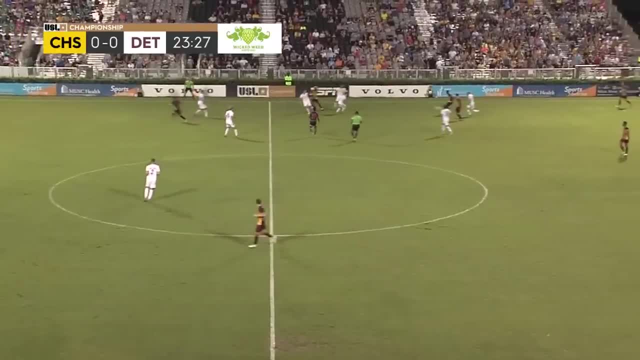 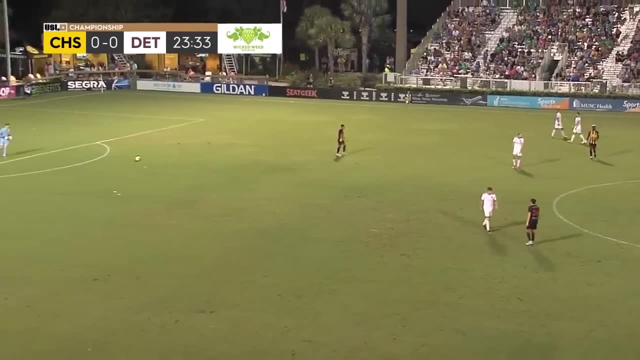 Rome was on. This is a great up back through type action here And I think you know it looks like Aiden's on. I think the ref was pretty quick to call that. I think that's a great, great run from. 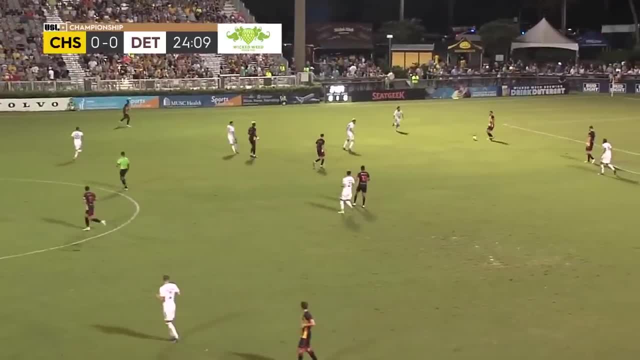 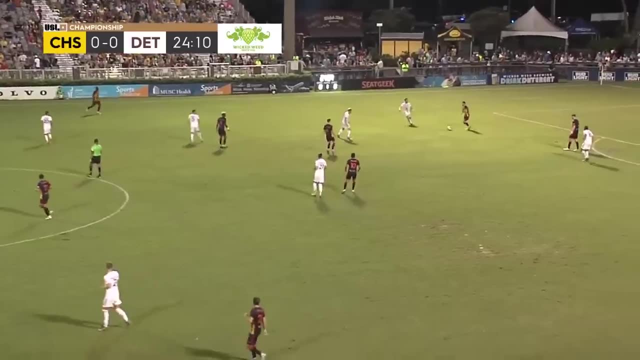 Aiden Apodaca. That's a great ball from Deezy. Unfortunate that it's off Receiving the ball now. lots of pressure coming in from this side looking forward. There's no clear passing angle. I kind of get myself in a little bit of a pickle here. 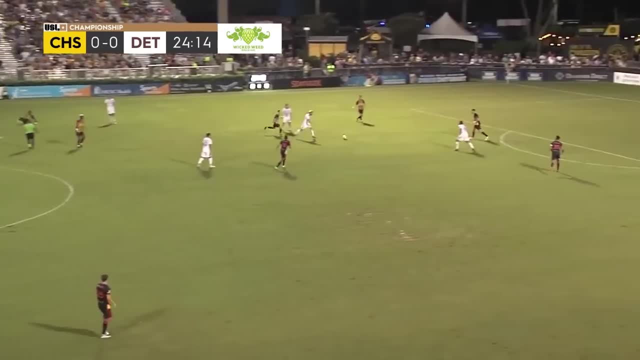 And then, with the outside foot, try to play to Deezy, my wing back, and he ends up getting fouled. but it's gotta be careful there. That was one of those. players was like: Ooh, I gotta be a little bit smart. back here Once. 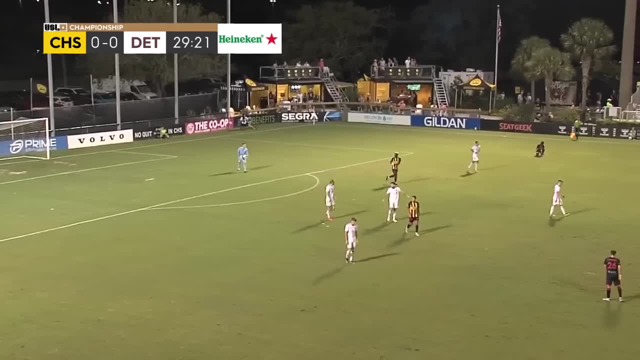 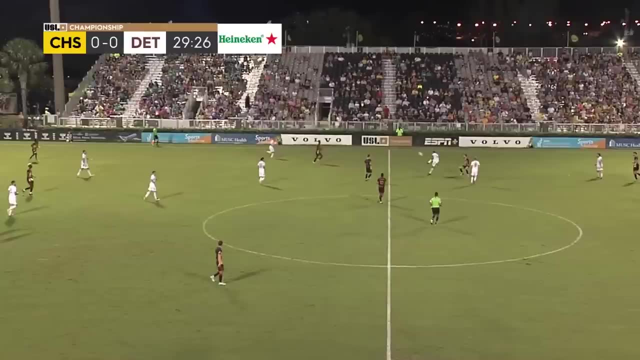 again just winning. the header. ball goes into Deezy, my wing back and then just dropping back a little bit in case he wants to play that ball back to me. Long ball into my guy, Batello Faz. I'm a little bit behind. I thought the ball was going to go a little bit further than it did, So I'm just. 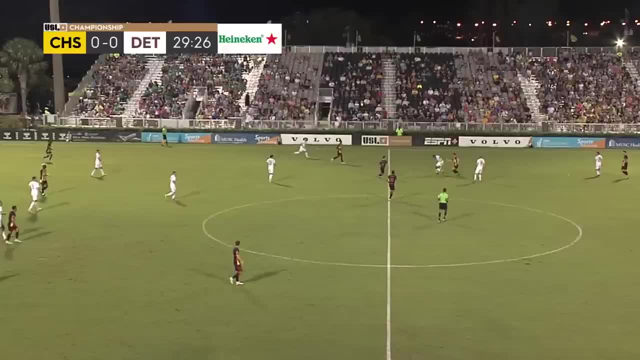 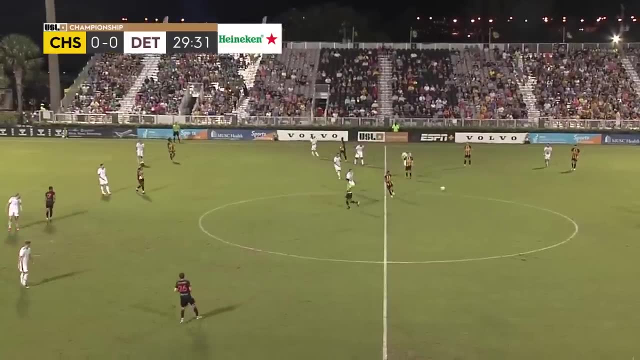 being careful in case he flicks this on and turns as he brings the ball down, as he takes a touch, that kind of gets stuck under him. I'm just kind of getting really close, initiating contact, sticking my foot in there and able just to poke the ball enough so that it can bounce out to one. 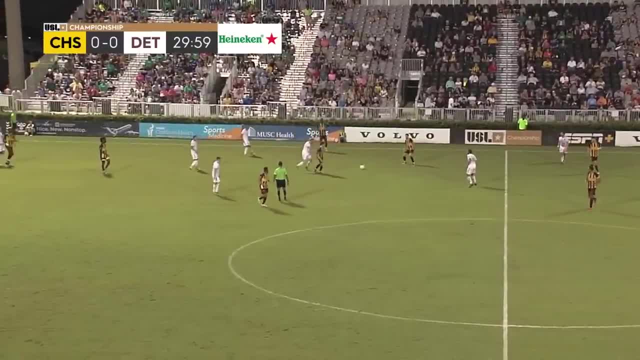 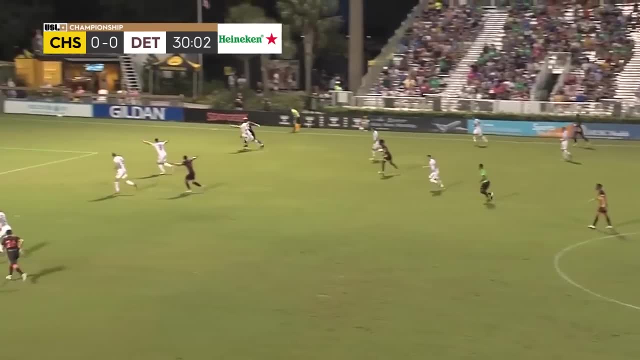 of my midfielders, Robbie takes the ball down, passes it right back to me. I see Augie in this, in this lane, beating these four Detroit city players. So I'm just going to open up play into Augie. I think that's a really good ball down the sideline And then Augie has a good ball into the. 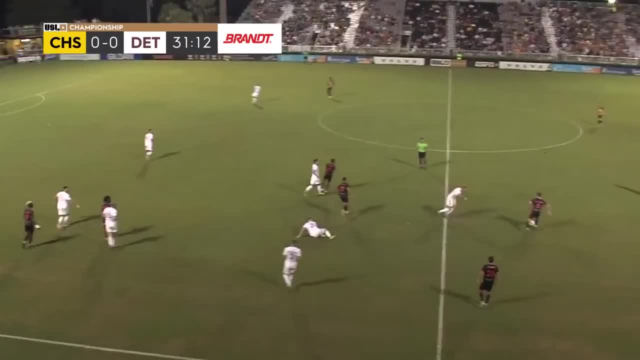 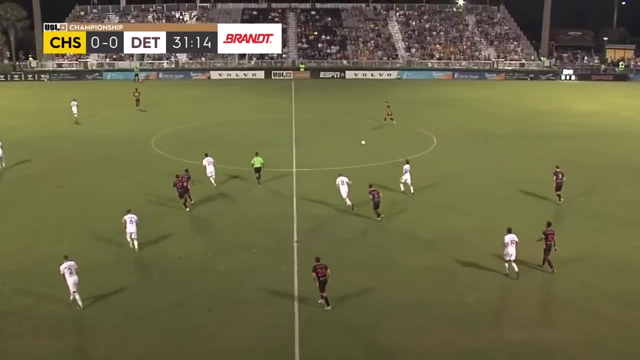 box. Just unfortunate that Charlie can't get on the end of that one. That's a good, great cross, Robbie, now with the ball. I'm just looking forward tons of space on this right side. You can see how much Detroit city compacts the game, but anyway, balls out to me kind of a rough touch there And 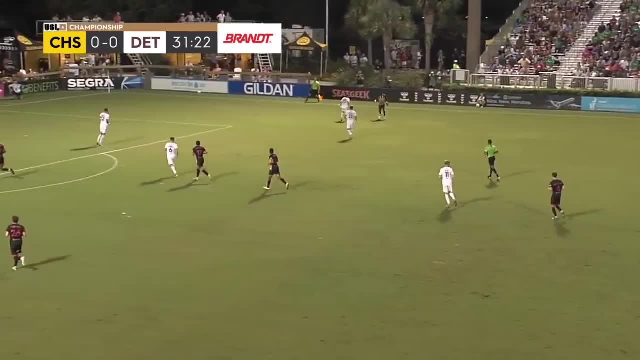 then a tough ball into DZ, but DZ is able to handle that, to be able to go one V one out here on the wing. Uh, Ugo Ferro, my goalkeeper, plays me out the ball. It's a little bit behind me here, I don't. 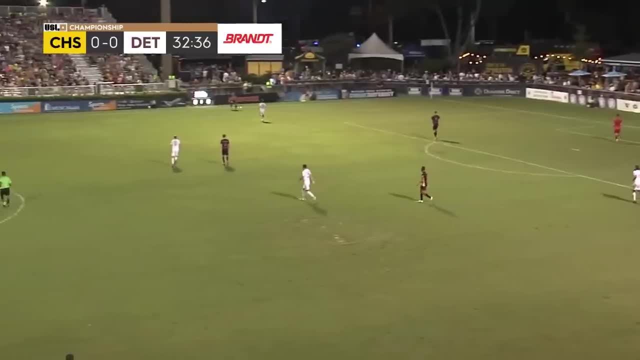 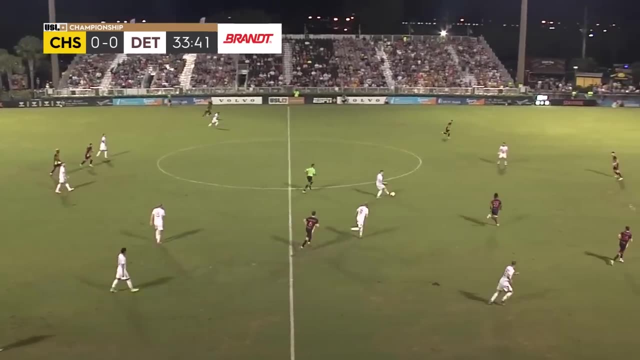 think I have the best angle, or I don't think that this winger starting to press me. I don't think it's the best decision to actually open up and drive down the line, So I take my touch backwards and then to play back in my center. back Now. a little counter attack here. We lost the ball. I'm. 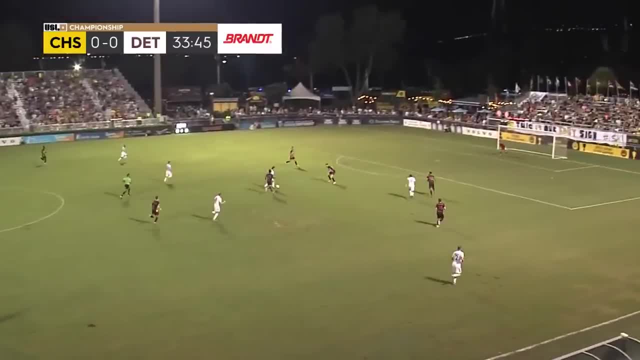 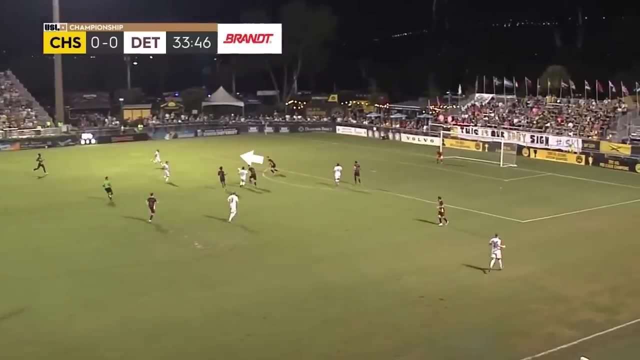 just recovering backwards, trying to delay This game. I don't want to recover too much, So I'm just going as far as AJ here, my left center back. I don't want to go any deeper than that, And then, as I get into position, I'm opening up my 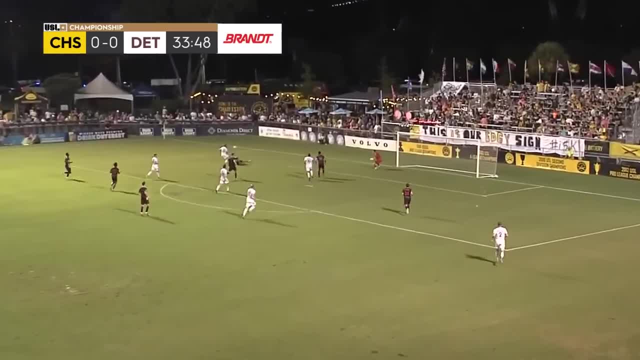 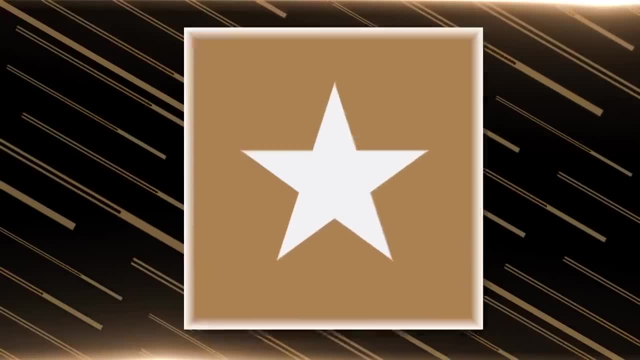 body turning around, So then I can face these two runners. good touch from the winger there, but I'm able to track that run and then slide as he crosses the ball. It's a tough decision, Like when you need to slide or when you just need to try to stand up cuz you think he's gonna cut it, But I think. 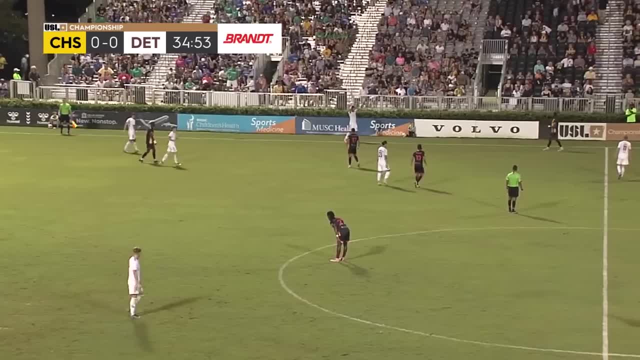 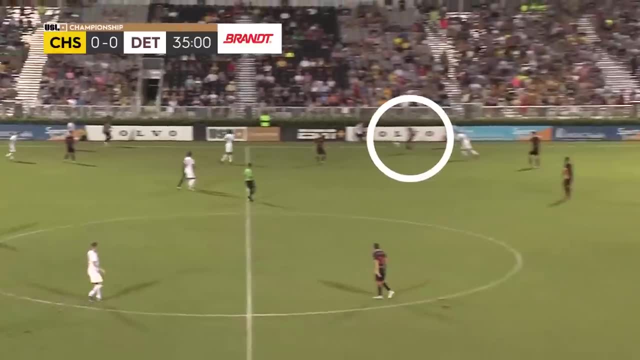 in this situation. it's a great touch. It's a tough situation on the counter. I think that's a good decision: to slide there and kind of expose Yourself, uh, in case he, even if he does cut the ball back, just stepping in winning the ball here. 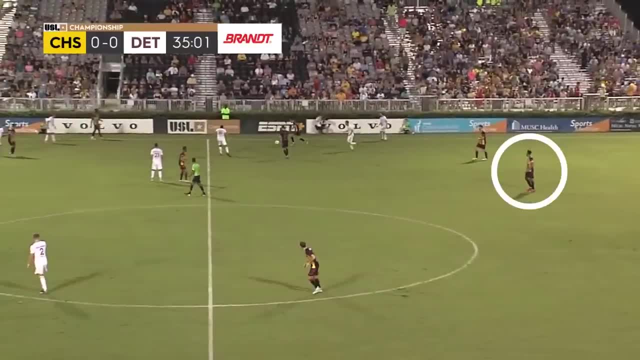 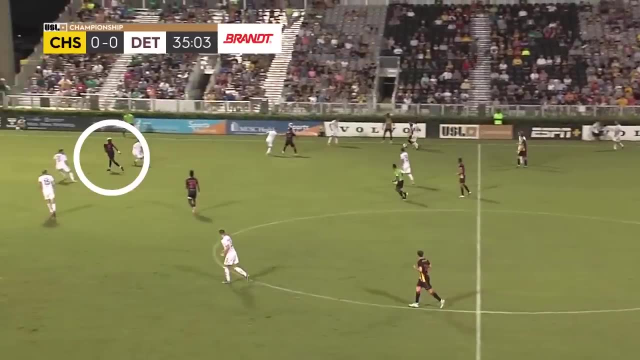 and then driving down the line, I think I could play into Robbie or even switch it out to AJ Patterson here. Um, I think that's a good decision by end up continuing to drive forward. Once again, Augie making a great run behind this center, back. I think this again is a good ball. I just 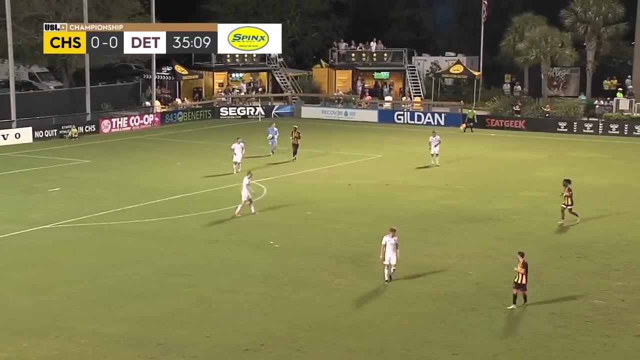 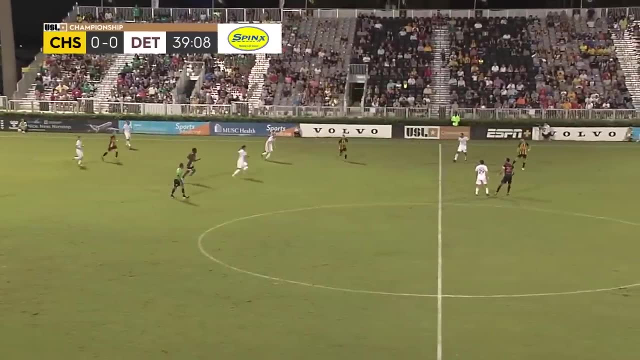 the execution needs to be better. Just hitting that a little bit too hard, easy for the goalkeeper to get that. So there's gonna be. I think again the idea's right, Just execution needs to be better. Uh, going up for a header there- missed that one- And then going up for the second header. 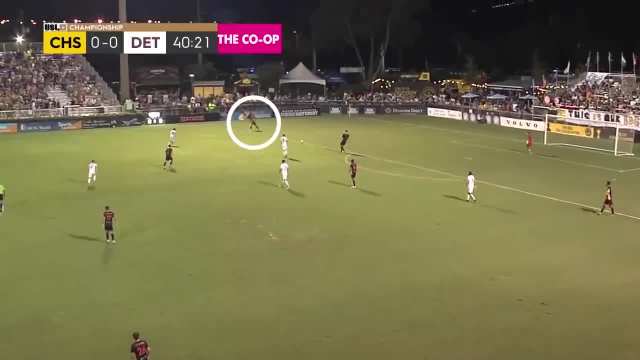 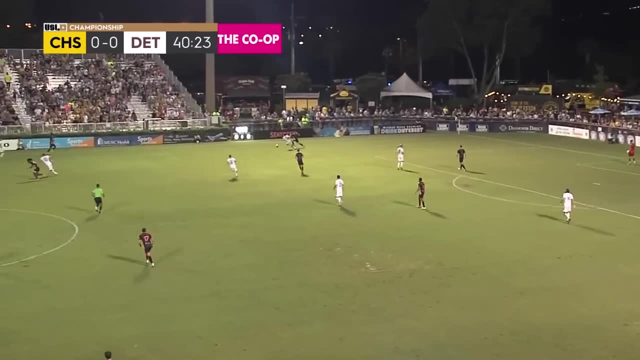 didn't win that one, but I did enough there for us to uh stop that play ball comes out to me from Pat Hogan receiving the ball. I think I can bounce into Robbie here. It's tough, There's a lot of pressure. I try to go wide, get a little shoulder to shoulder contact. Um, uh, it's just. 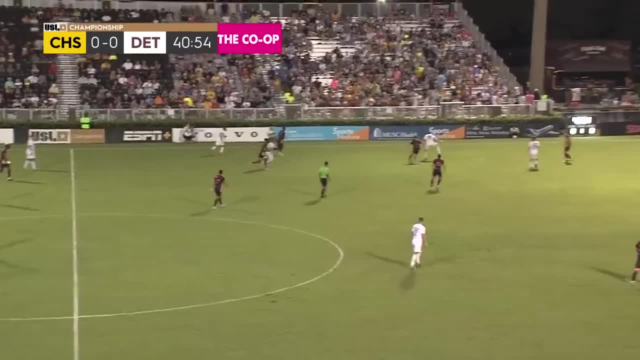 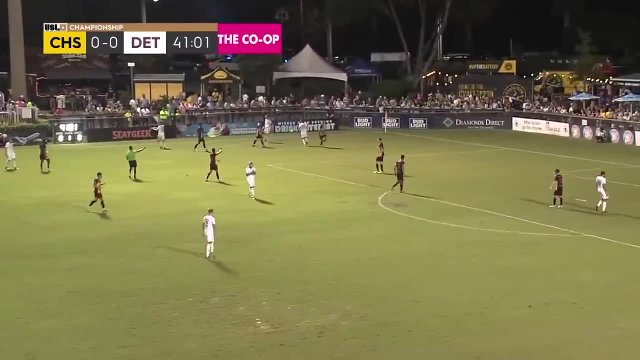 good pressure, I think, from Detroit city, but I think, as that pressure came in, calm down a little bit and try to find that central mid, and then Robbie's pressuring out. this winger just come over. make a tackle out on me, though. for Detroit city FC, Now here, just another free kick, very. 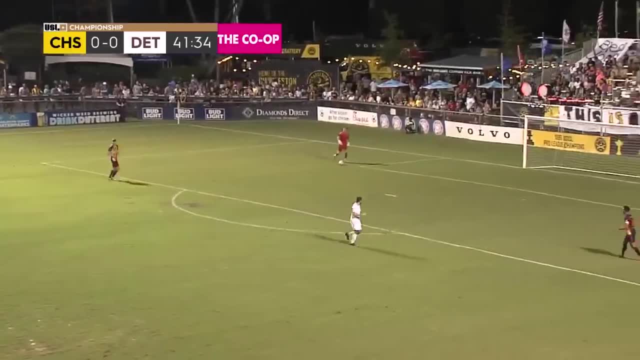 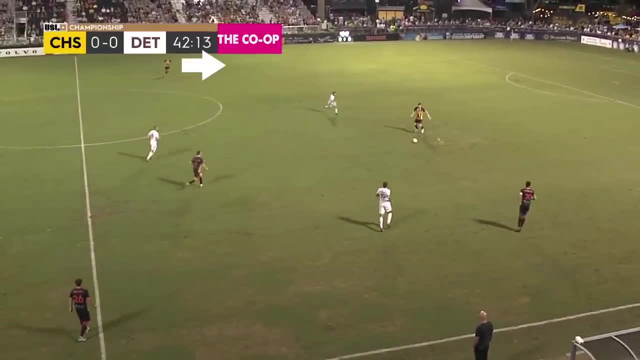 very deep in our own half. So I'm just gonna play back to Ugo, since they are not that high up the field, And then he can kind of make the decision here Now. here, the reason why I'm not flying back to create a good angle, a good passing angle for Pat here is because this is a good little. 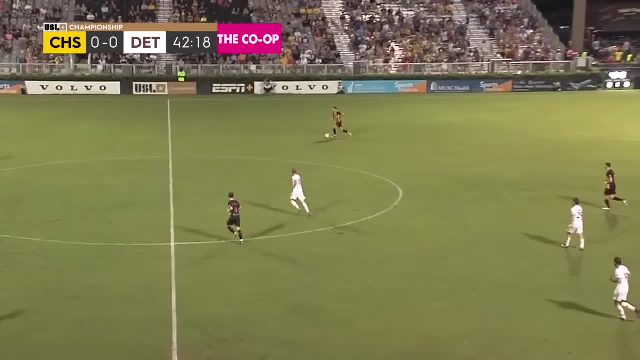 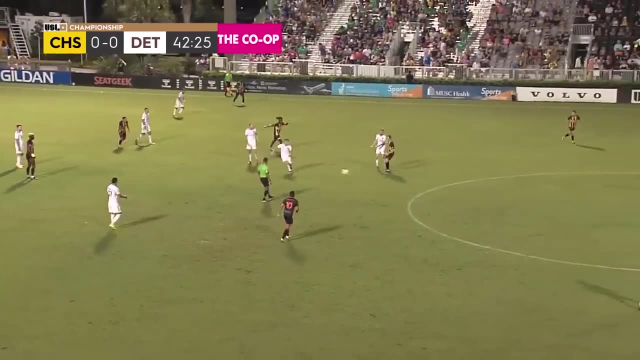 combination. I know that ball's gonna come into Robbie most likely, And then I wanna create a passing angle for Robbie instead of for Pat there. Now I'm gonna drive forward, play into one of our tens, unfortunately lose the ball again and now we have to recover. And then here this to me: 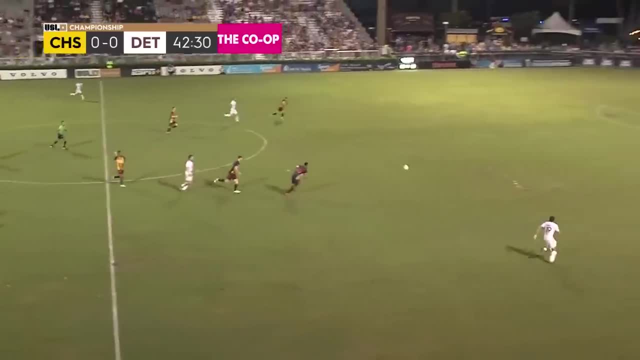 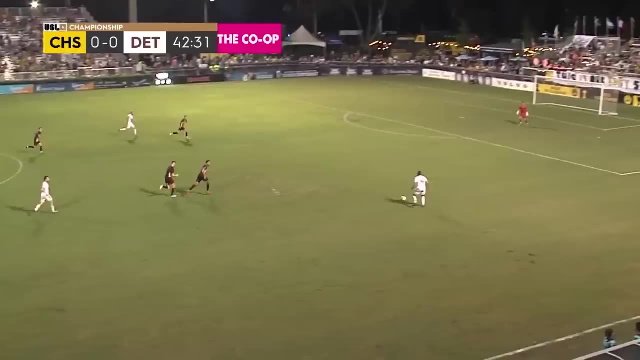 this might be a bad angle, but it looks about five yards off side. Uh, but good, recovery run I'm. I'm not just stopping and raising my hand. I did raise my hand, but I'm recovering, first sprinting back And then, as soon as Patel Fas takes this big, heavy touch here flying in, I know I can win this. 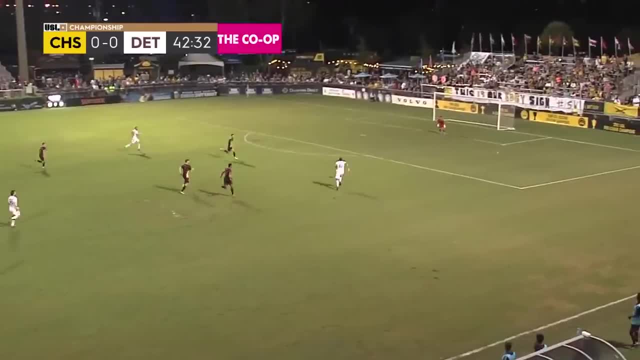 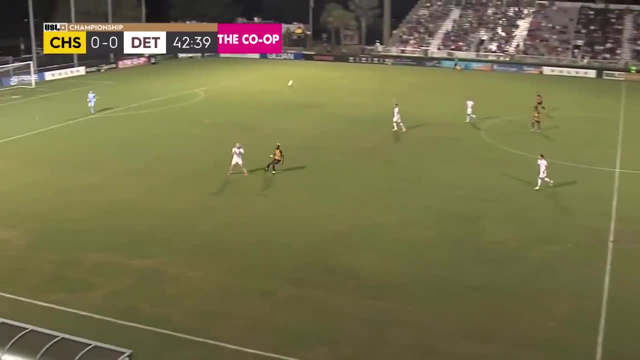 I know I can get there first. So I'm trusting that, trusting my instinct, flying in and just uh winning that ball and uh moving forward. Now I'm just gonna clear this ball up. try to find uh Augie or striker, because 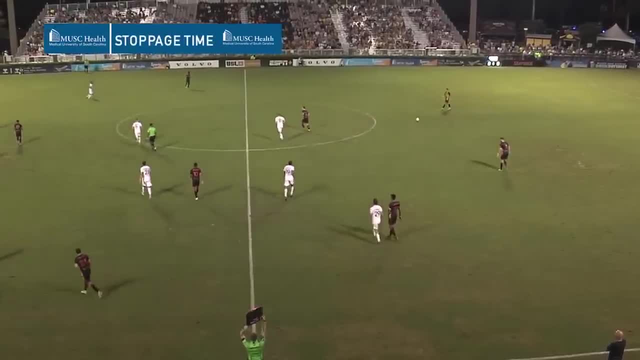 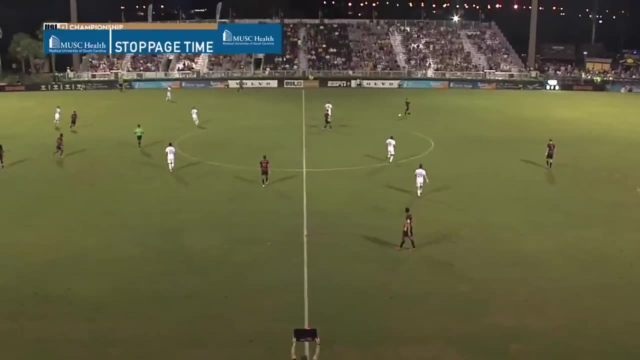 we're so out of position. It's kind of a dangerous play. I don't wanna just go turn around and lose the ball too quickly Now. receiving the ball here, tons of time looking forward. I'm not really seeing what I want out on the right side, So I'm gonna put my foot on it, kind of chop it back and 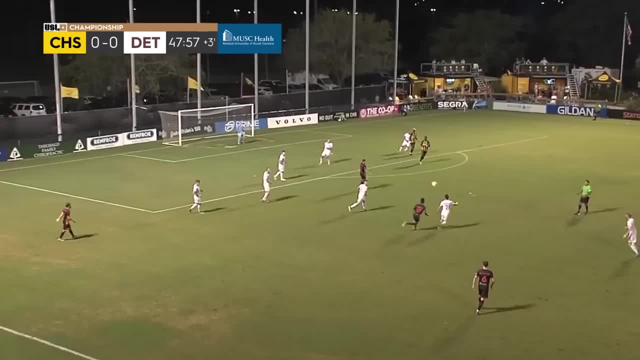 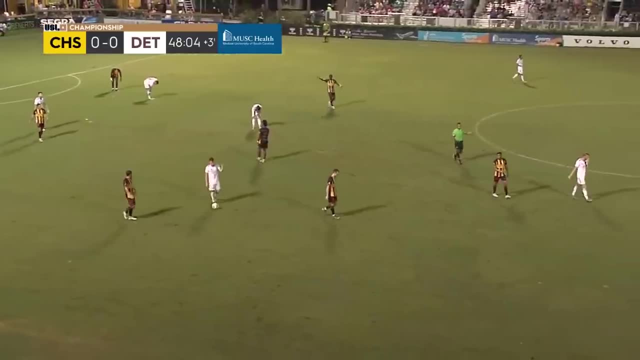 just play right into Robbie and tell him to turn and face forward. who ends up playing it out to DZ? And then here, Detroit city FC with the ball, but the last couple seconds of the first half, referee decides to end the half there. 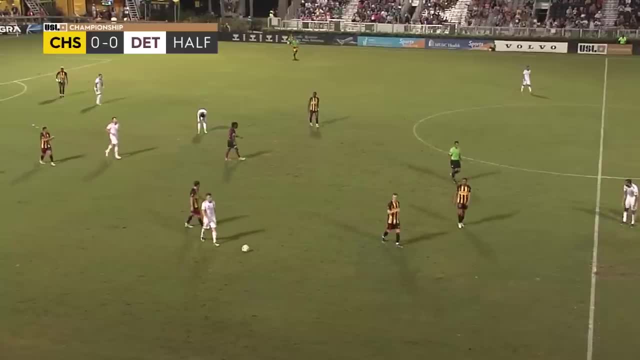 So Yeah, Yeah, Yeah Yeah, First half: nil, nil, um, defensively, you know, as a center back, I'm I'm very happy with this first half because I don't think Detroit city FC had a shot on goal. 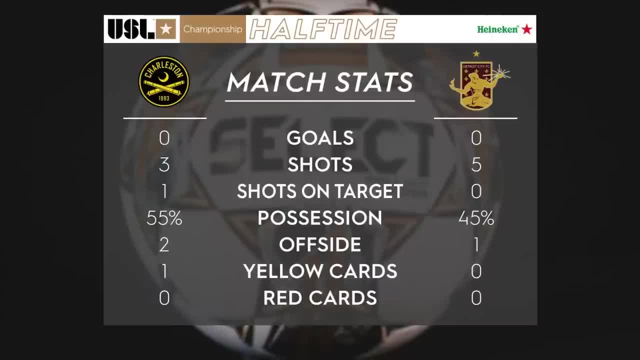 Um, so for 45 minutes, really really happy with that. However, you know, looking forward are three shots and one shot on target is not much better. So we did have a little bit more possession, but they ended up having a little bit more efficiency in the final third. 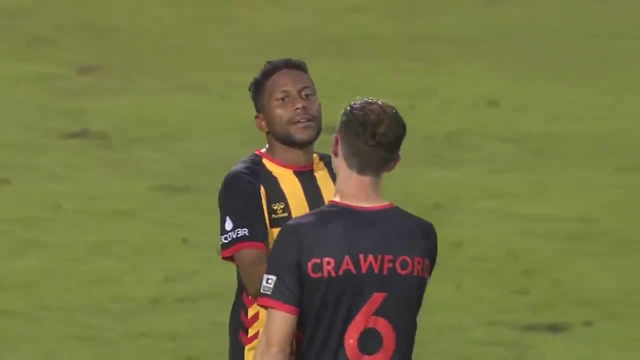 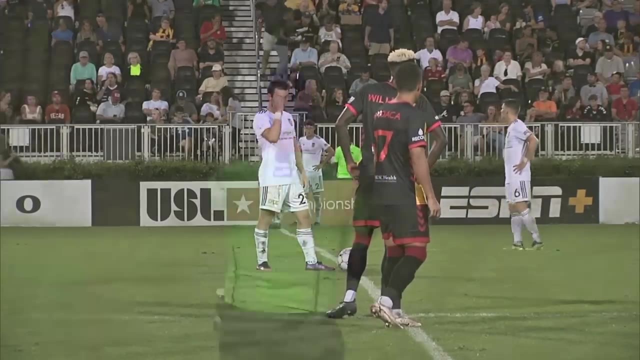 getting a couple more shots than us. So not the most thrilling, uh, end to end action, but I think our possession of the game, our ability to manage the game And then just defensively, our team defense was really really good that first half. So anyway, here is the start of the. 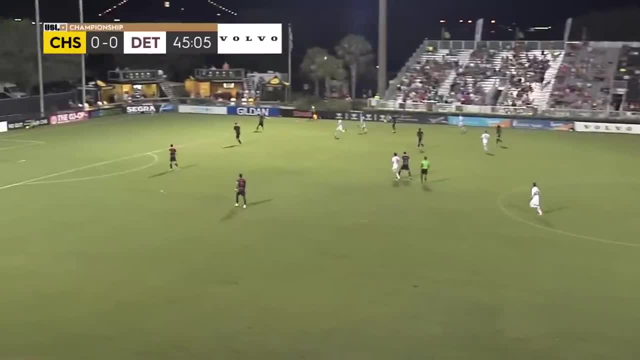 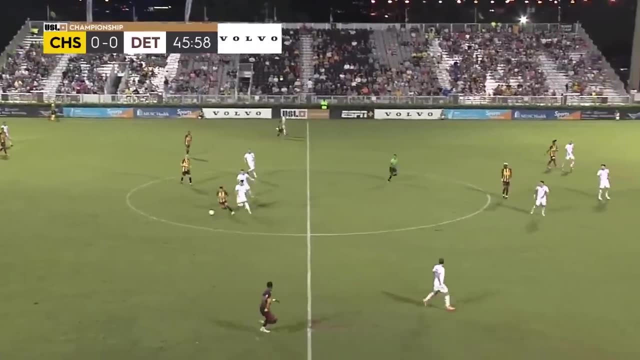 second half. Detroit city FC starts with the ball now and they go long to that far side of the field, ends up going out for a throw in, And then here is going to be my first touch of the second half. So Aiden Apodaca has the ball, plays it out wide to me. I could drive forward, but we just won. 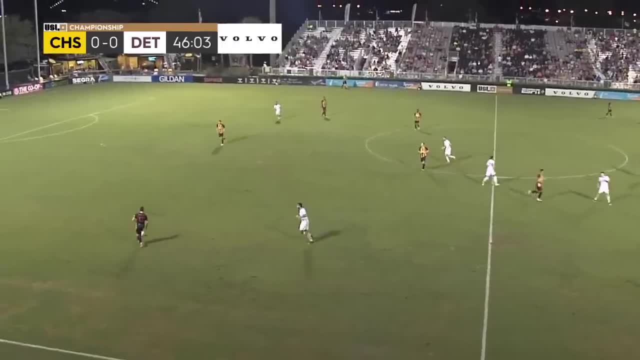 this ball after about a minute of not having it, So I'm going to cut the ball back. little Cruyff, turn just open up And I think Here. I think I could take one more touch inside and then try to find Romario Piggott here Instead. 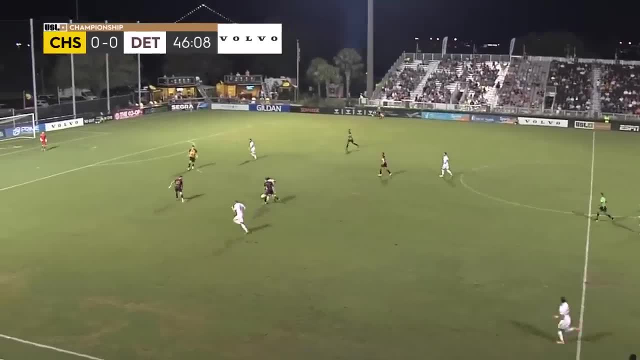 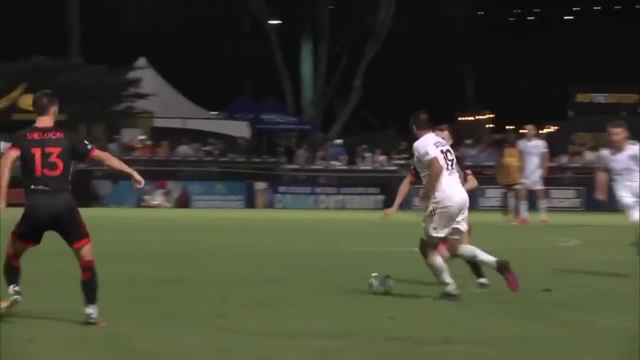 I kind of play into Robbie Crawford a little bit of a heavy pass. He has a little bit of a heavy touch and then he decides to do a tactical foul there, pull him back and take the yellow card to stop that counter. So, um, yeah, I think I could have played. I think it would've been a. 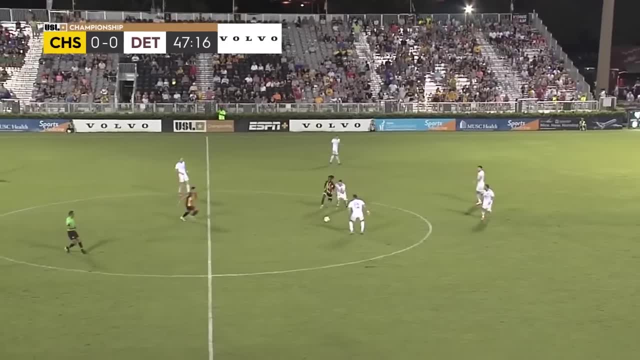 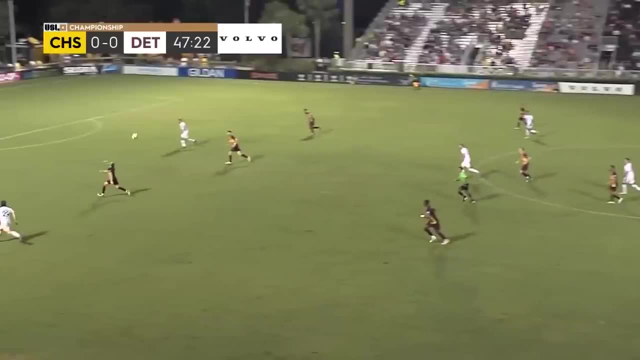 better decision to Kate: take one more touch inside and play to Roma there. Uh, and now we have the ball end up losing it. A little counter attack here from Detroit city pops over my head, difficult angle right over me. I think if my body orientation was a little bit better I could head this out. 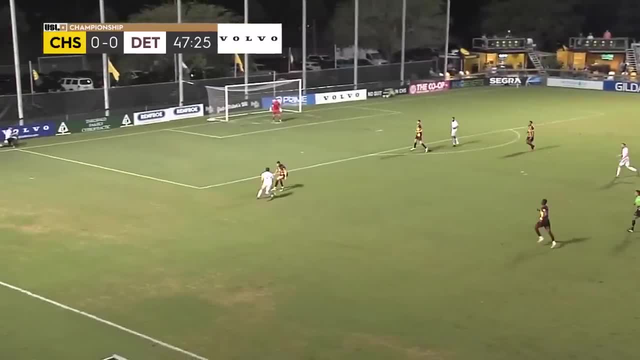 but that's a tough ball. I don't want to stumble over my feet or just miss the ball completely And then have hoping to be able to go one V one against my goalkeeper. So anyway, uh, decided to stand him up. I should do a little bit better of a job forcing him wide here, hoping I was still. 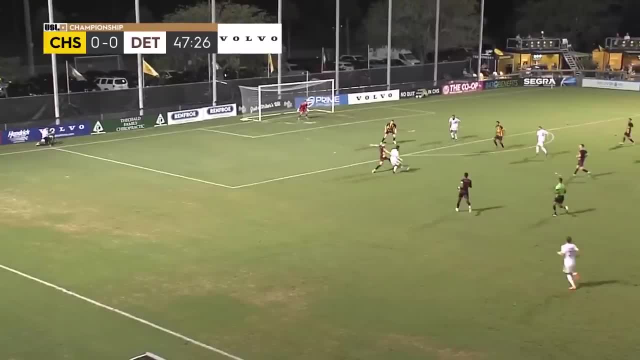 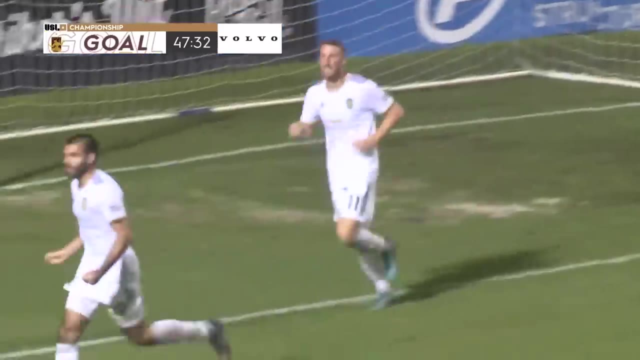 able to cut inside. I'm still in a good area to block the shot, But the problem here now is that our back post area, back shoulder, were not sorted here, So I think the AJ could be here in a line of contact with Pat or if. if Pat wants AJ to step up to that center guy, Pat needs to then follow. 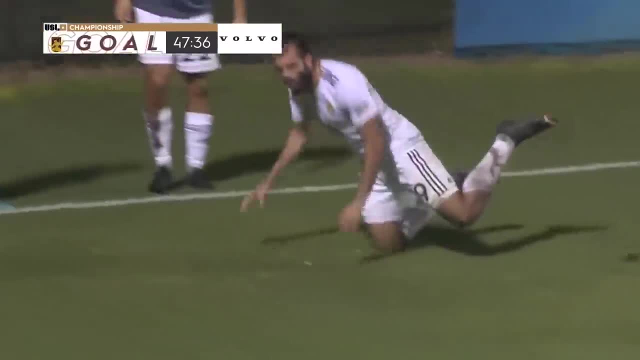 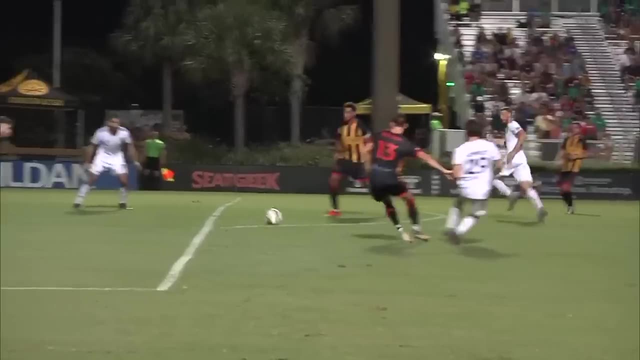 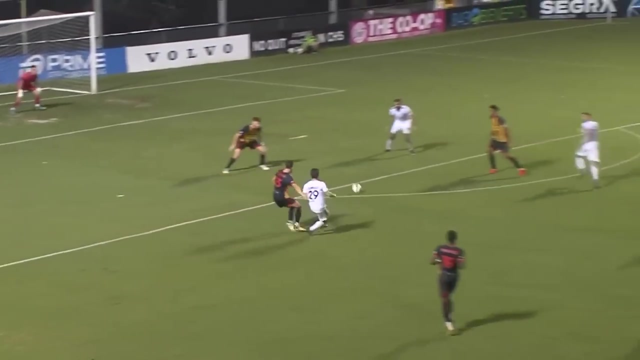 Botello Fahs the guy who scored. So it just needs to be a little bit of communication back there to sort it out. Personally, I think, if I think it's smarter of AJ drops back with Pat um instead of just one view, one all over the place, but it's, both can work, We just need to be on the same. 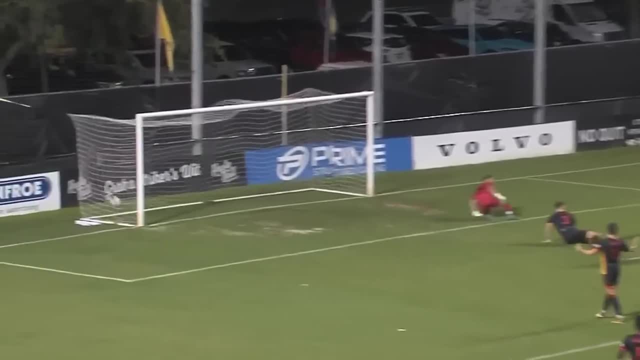 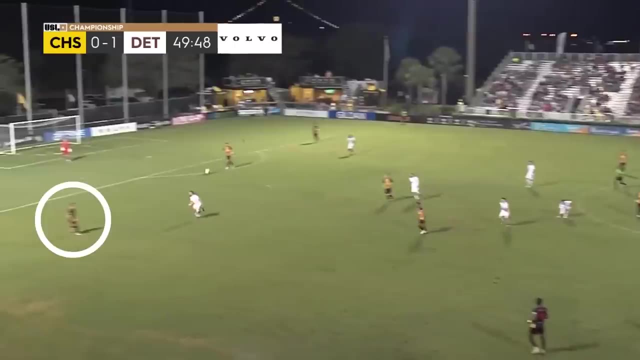 page. We're on different pages here And then we end up suffering because of that. Anyway, here's my touch after the goal. ball is going to bounce all the way down to me. I know I can win this, but I need to take my touch in front of Hopeno here so I don't get crunched for a tackle. so I'm going to. 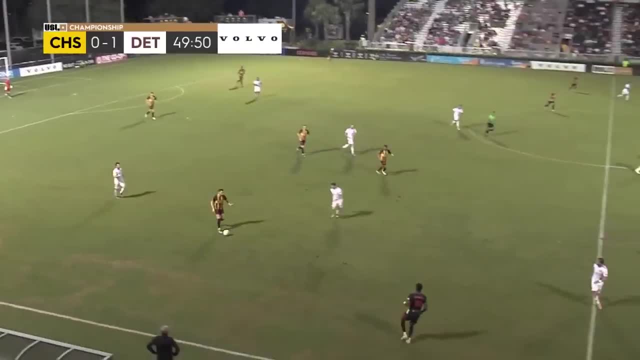 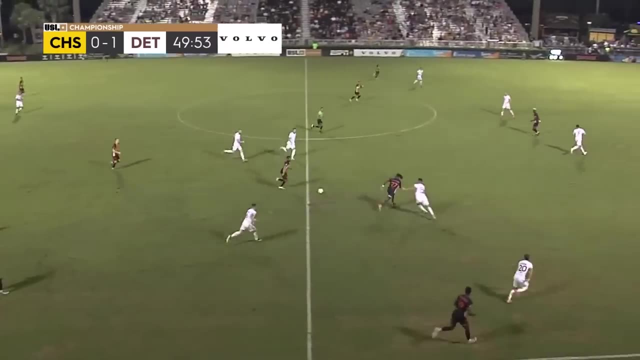 just take a touch right in front of Hopeno, drive forward and honestly I think I make the wrong decision. but it works out. I think I should play into DZ and DZ can bounce it to Romario Piggott. here I end up just cutting the ball into Roma. it works out, but uh, got to be careful there because 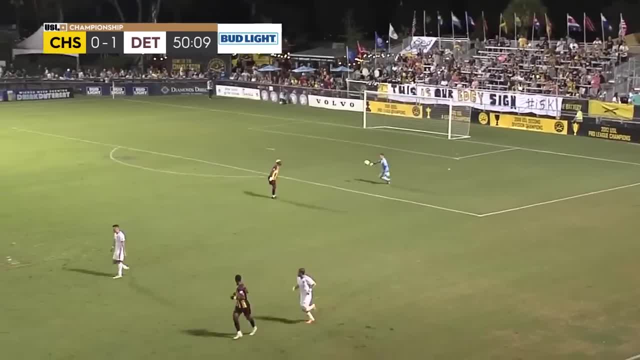 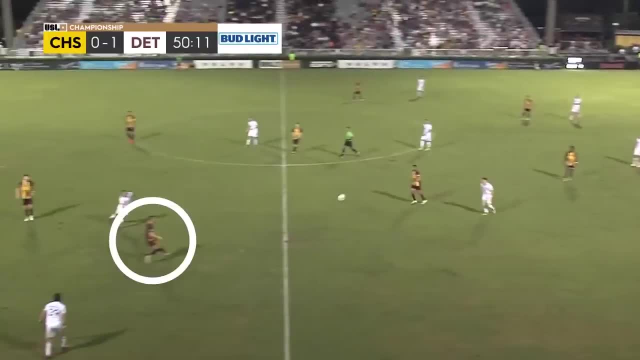 if I play that ball into a Detroit City FC player. I mean, I'm one of the last guys back there and it could easily lead into a goal. now ball comes into me. I try to trap this ball down so I can play forward. I think it's a good idea. just the touch isn't there. just the touch lets me down a little. 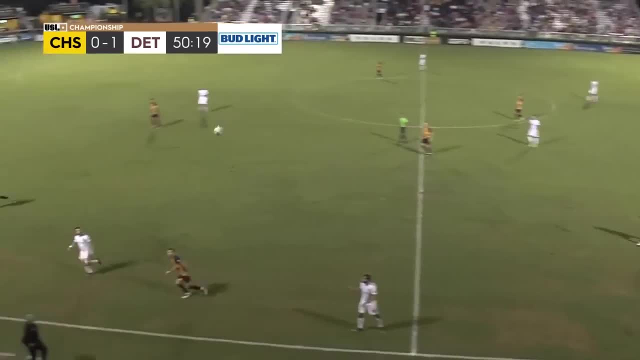 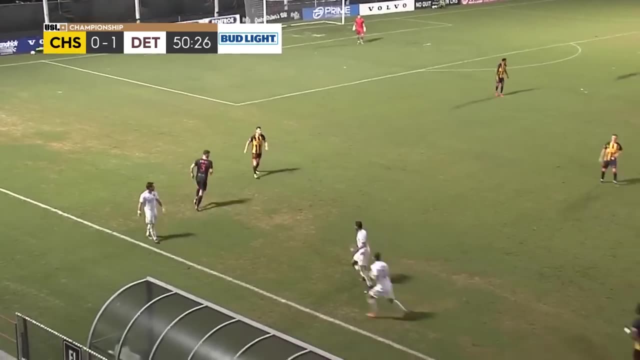 bit the ball's a little bit behind me and then Botello Faz is able to uh win that, and then, uh, they play down the line. we end up winning this. me and Pat do a good job just to clear this out of danger and get back into position position, but uh, yeah, just need to do a little bit better. 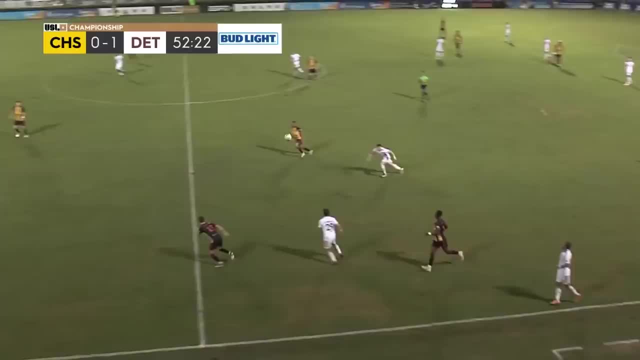 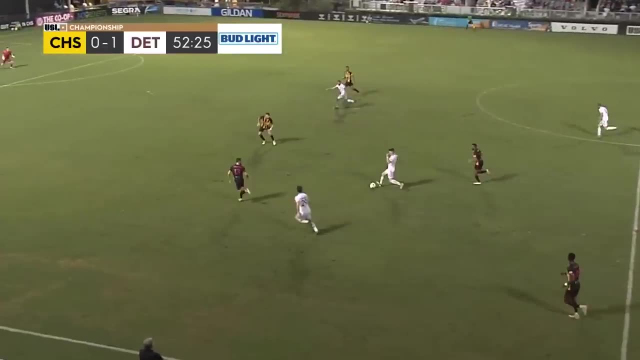 execution on that touch now here. this is a complete miscommunication for me and Roma. I thought Roma was going to get this ball, Roma thought I was going to get the ball. we end up both leaving it, but however, I mean, it's still okay. it's still okay at this point, and then AJ. 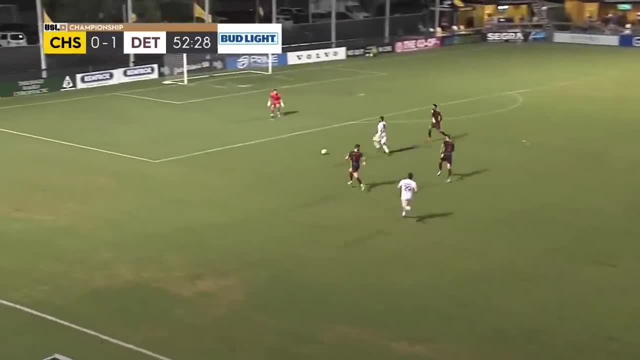 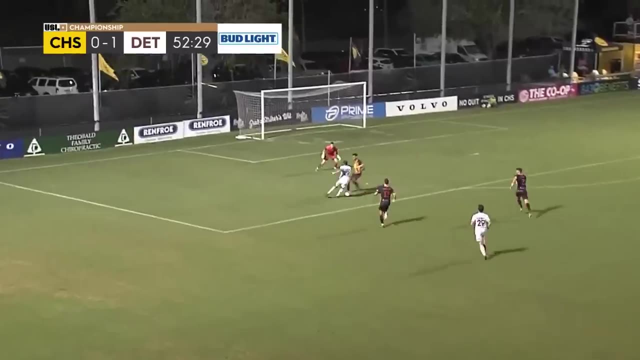 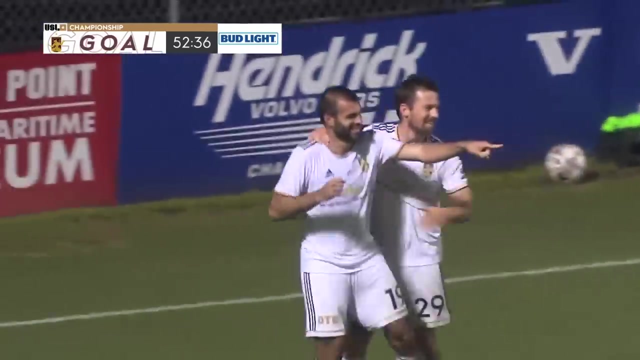 lets Botello Faz make a run in inside of him without tracking and then flies in across Botello now without making a tackle. it's a great cut from Botello and then he's able to just hit that into the back post. so lots of little errors that led to that goal initially starting for me and Roma. 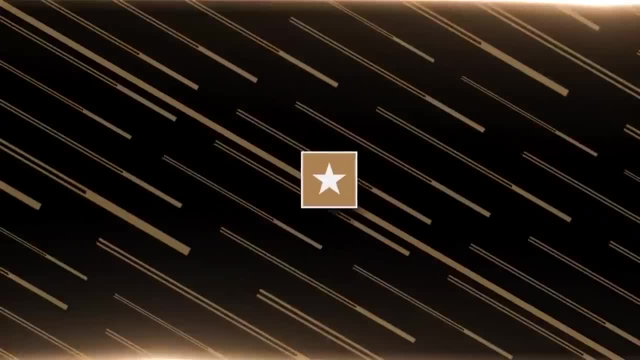 both thinking the other person was going to get the ball, and then he's able to just hit that into the back post. so lots of little errors that led to that goal initially starting for me and Roma to win that ball um, right here. so it's a little deflected. it's kind of hard to judge from that. 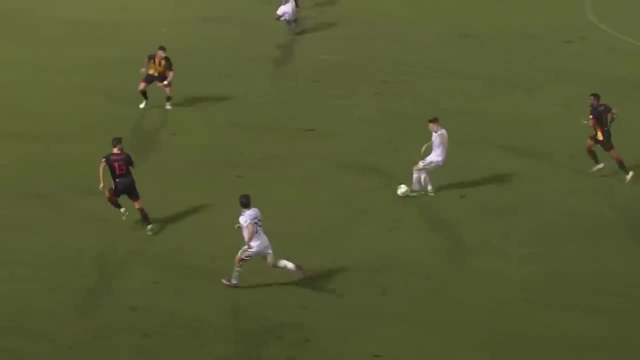 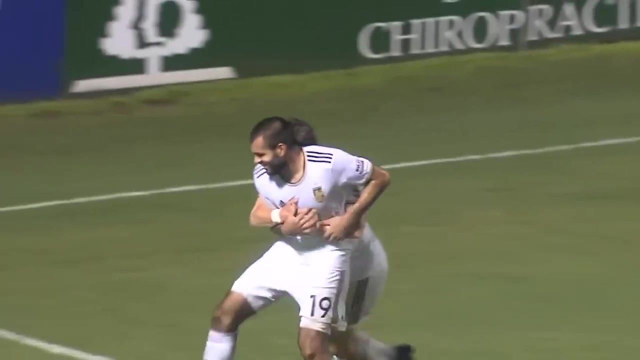 deflection but we both think the other person is going to get it. and then not tracking the runner here, and then over ambitious on the tackle, and then you know when you do that, when you have three mistakes like that, a good team like Detroit City is going to be able to capitalize on it. 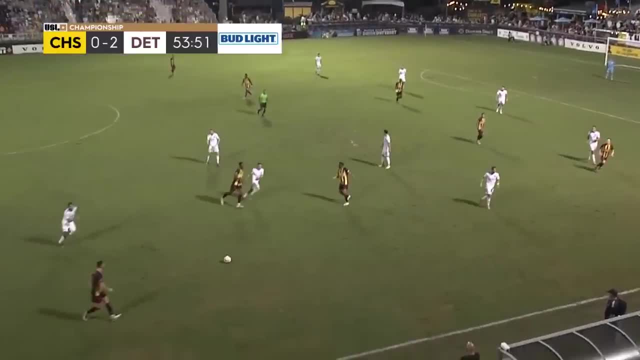 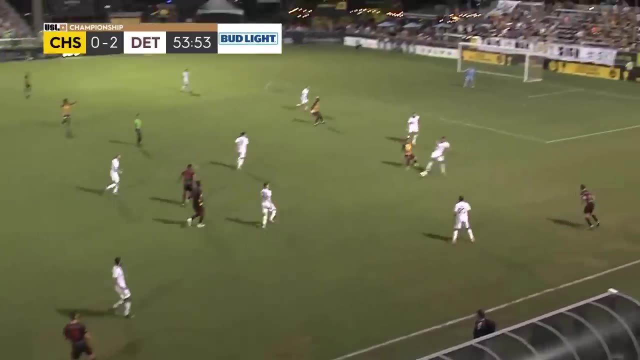 now, 54th minute. now ball comes into me here looking at the film, I did not see this at all, but I think I can play Romario right here. I don't know who that is I should play. oh, I think that's Ayo. I should be able to play Ayo in here. end up trying to play into Aiden Apodaca doesn't work. 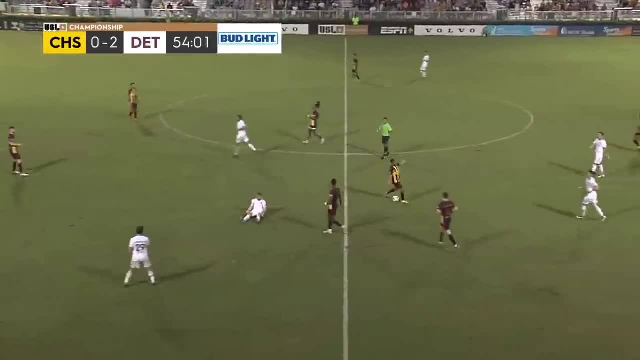 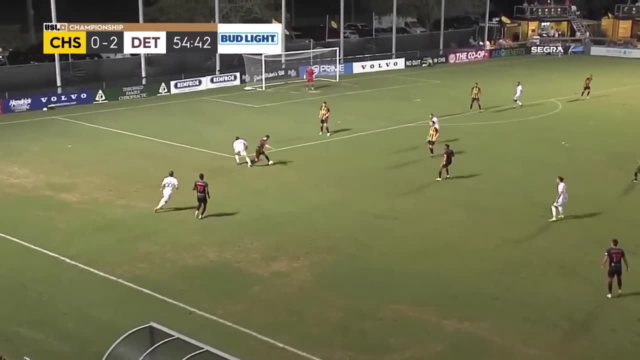 out and leads to a little bit of a counter-attack and Roma has to take the tactical foul. but yeah, it's easier to see passing angles from over up on the bird's eye view. good tackle here, able to win the ball from Hopeno, and then again this is like one of those things that instinctually it kind of 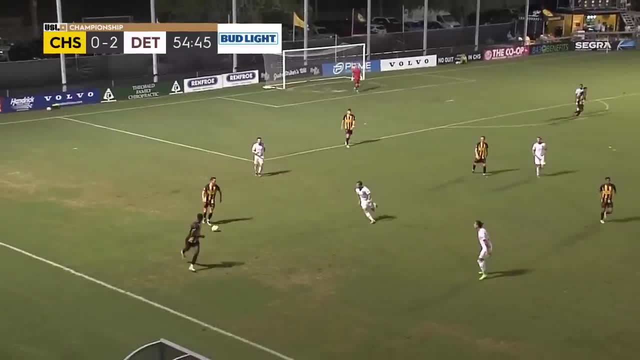 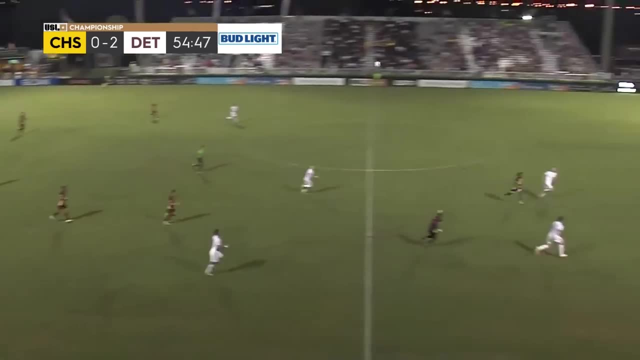 just happened. but I'm not saying that you should try to do a croqueta here in your own own half, but able to just get around that player and look forward now and then I'm trying to see- I see a runner, I see Ayo Flanagan making a run behind. try to play him that ball, but just don't get. 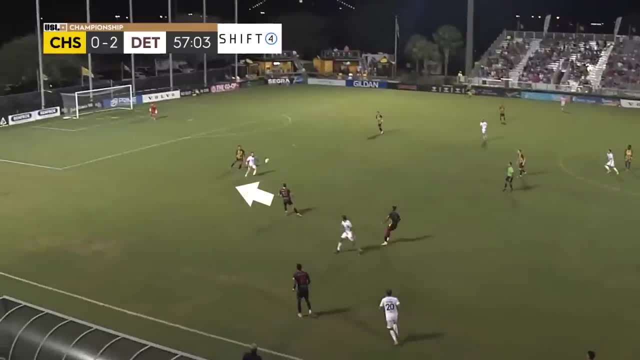 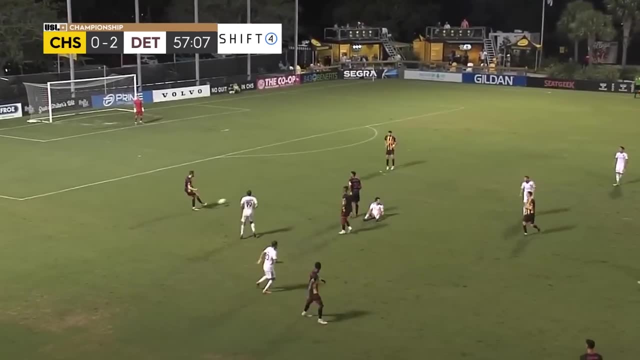 enough on it now. as this ball goes over my head, I need to cover him behind in case AJ Patterson now would get beat. so I'm going to fall back, get him behind. we end up winning the ball, able to create a passing lane for Booth. I'm going to play it over to Pat now and we can keep possession. 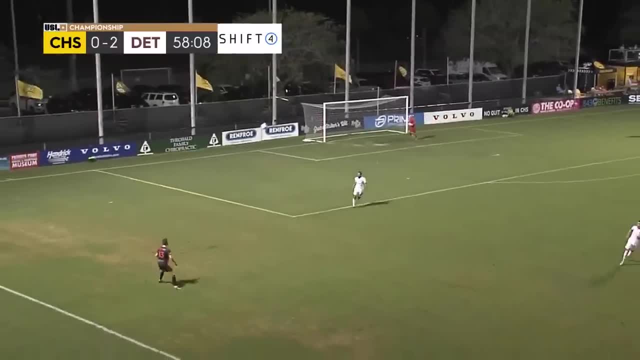 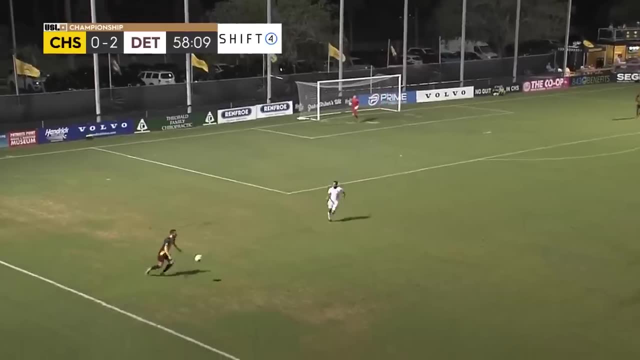 of the ball and look forward. now Ugo Ferro, my goalkeeper, finds me with a great ball out. I'm going to open up. I've already checked my shoulder. I know I'm free down here, so I'm going to open up and then try an entry ball into Mauro Cicero kind of the winger on this side doesn't end up coming. 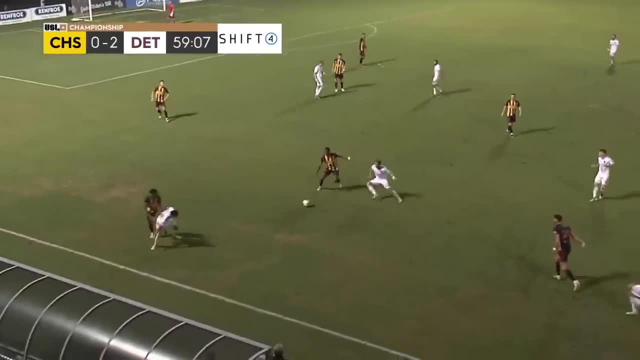 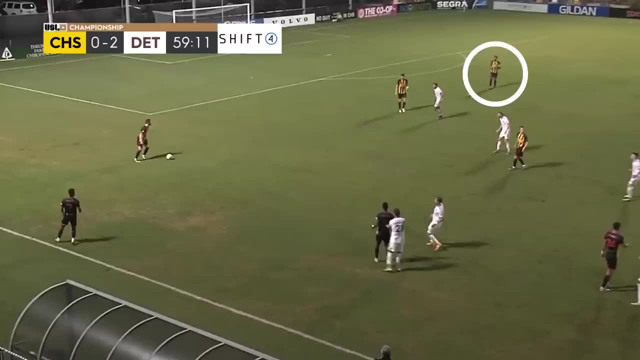 out, but uh, but we end up getting the second ball and able to do a little bit of a counter here. now we win the ball. Deezy plays me back. I got tons of time. now I'm looking over this far side. I think AJ is a little bit too close for me to try to switch it over to this far side, and we're kind. 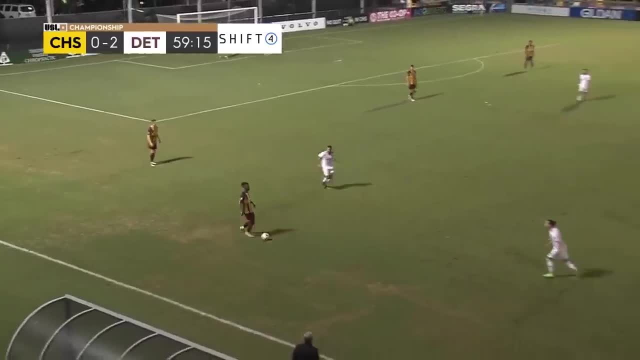 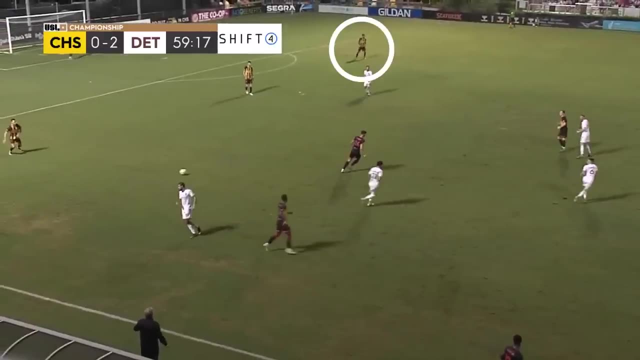 of marked up all in the middle. so I put the ball in the middle and I'm going to try to get the ball to play it close into Booth. Booth drives forward a little bit, plays into Mauro, who plays it right back to me, and now we're spread out and now I can find this opposite side. you can see AJ's in. 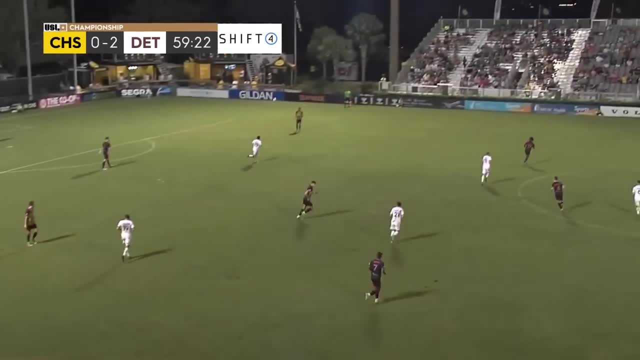 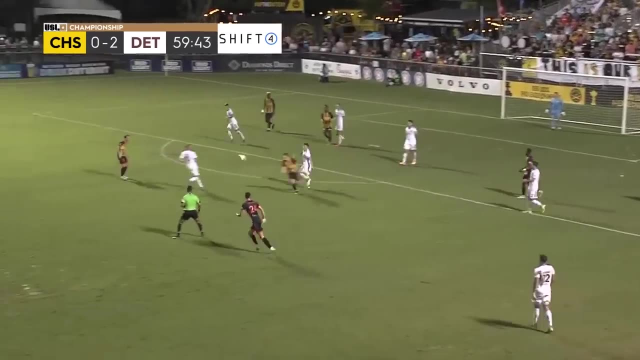 a better spot now so I can take my touch, look over and then find AJ Patterson with that switching pass over that far side. so just a couple passes to draw them in and so that we can expand and then we can switch. ball comes into me just going to take the touch down. play out to Charlie Asensio. 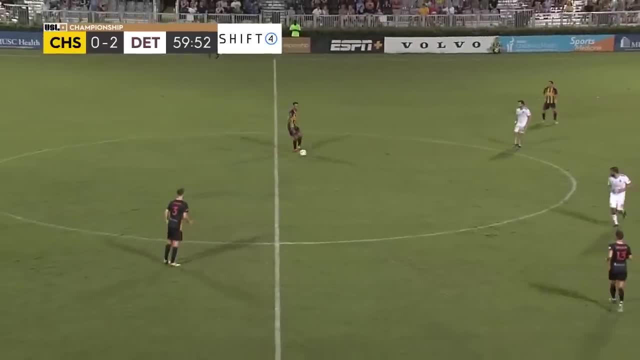 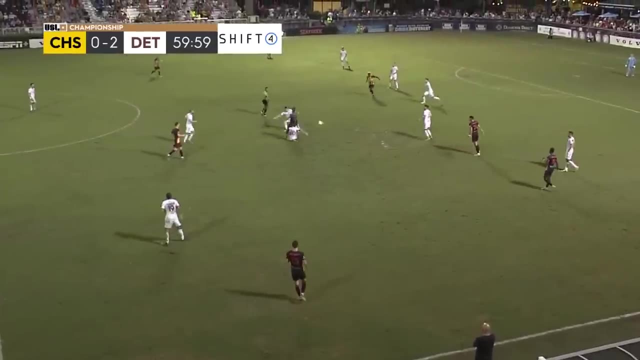 my left wing back and then I can kind of drop and get into a better position for for being a right center back. so now Pat Hogan, center back, has the ball, plays into Booth who takes his touch inside Booth, drives. unfortunate not to find Augie, but back out to Pat and you can. 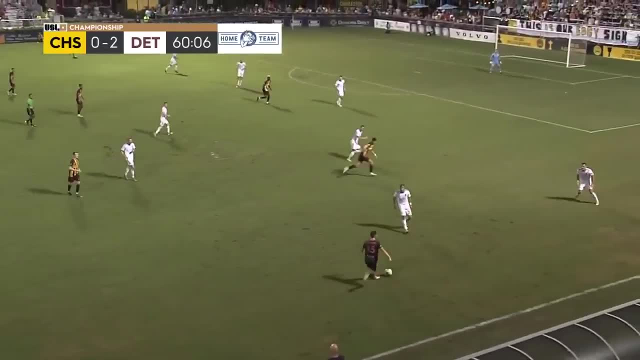 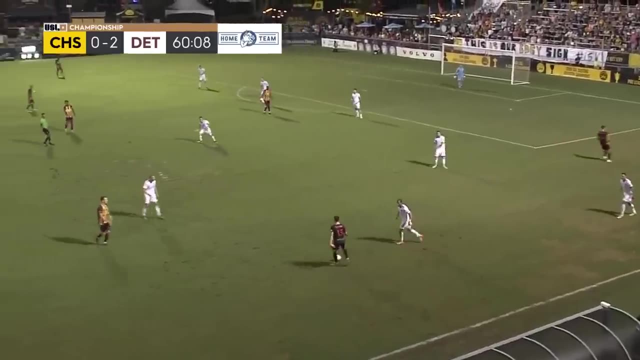 see my positioning. I'm kind of cheating, I'm kind of standing in front of their, their striker, almost as like a right fullback here. I think this would be a good ball to chip over the top of tomorrow and behind, decide not to do it, cut inside, play into Robbie and then get out of his way so he. 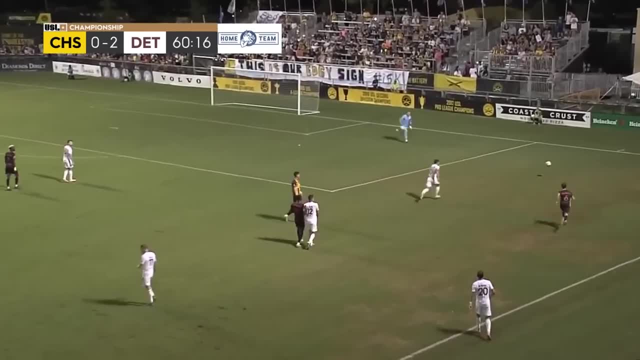 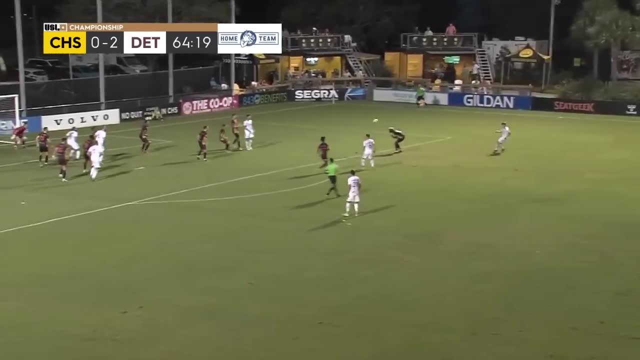 can drive forward. uh, who tries to find Mauro? but Mauro's already off from the run he made. when I hit the ball crossed in the box from a corner, kick just winning that header and then getting back in a position trying to organize inside the box. we do a good job- just to stop all of 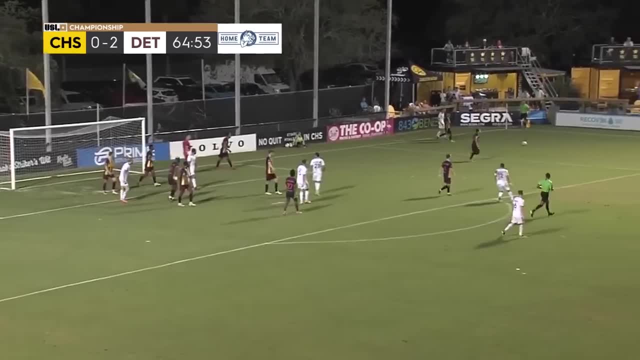 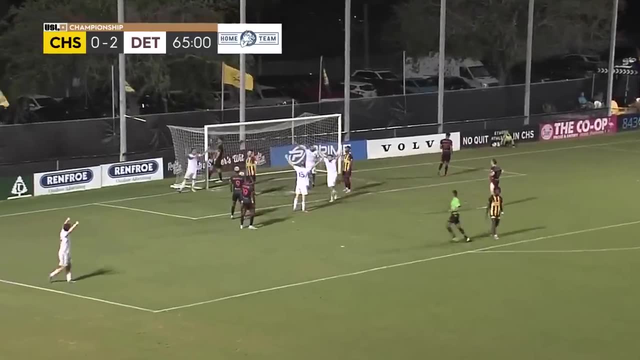 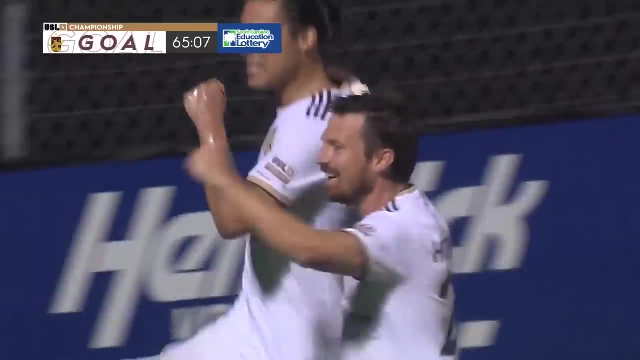 the attacks here, but then out for another corner kick once again. then from this corner kick, ball's getting played back, crossed in and then a lot of mistakes, again leading to a goal. a lot of mistakes, I think. I think Augie thought I was going to go up for the header, I thought it was over my head into. 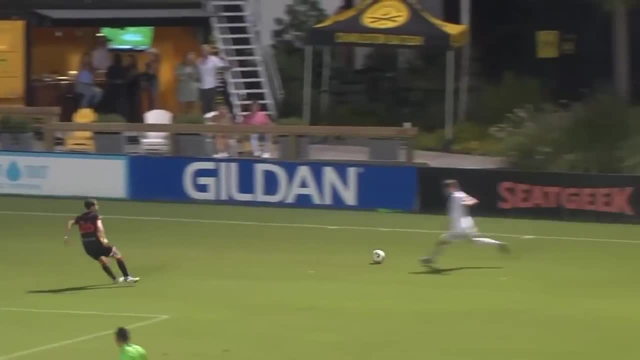 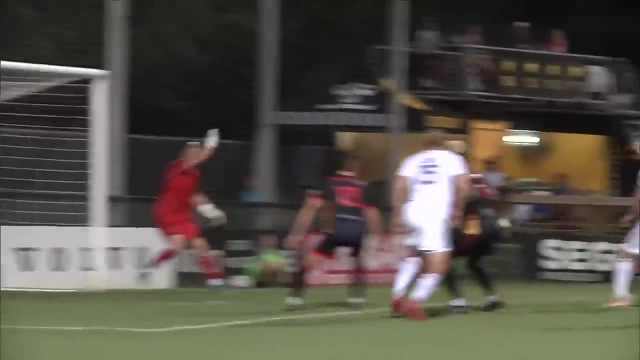 Augie's man, and then I think Augie didn't challenge for the header there and then I think, even though the Detroit City player wins the header, I think we should. I think Ugo's got to hold on to that there. so lots of mistakes here and uh. 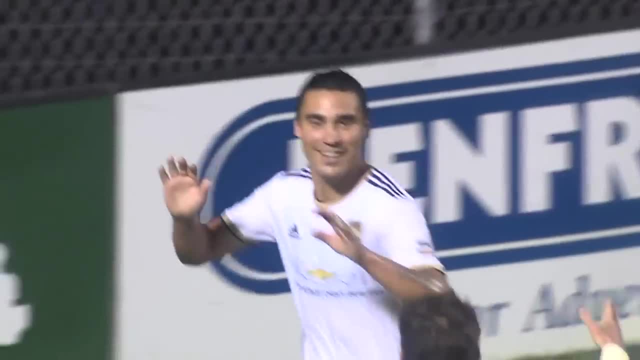 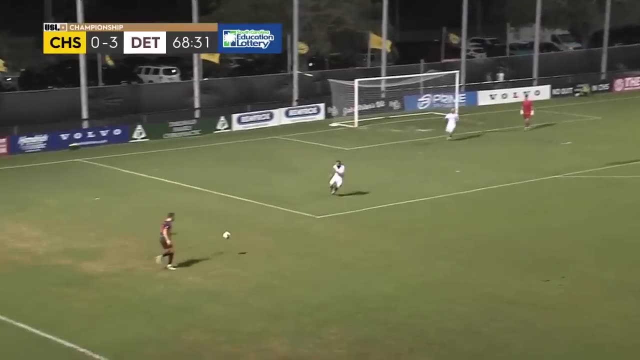 ends up leading to their third goal of the night, which is, uh, frustrating. it was very frustrating to watch this back. we'll go with the ball. once again finds me out now receiving this ball. you can see botella flaws the angle he's taken to pressure me. so I'm going to drive forward and 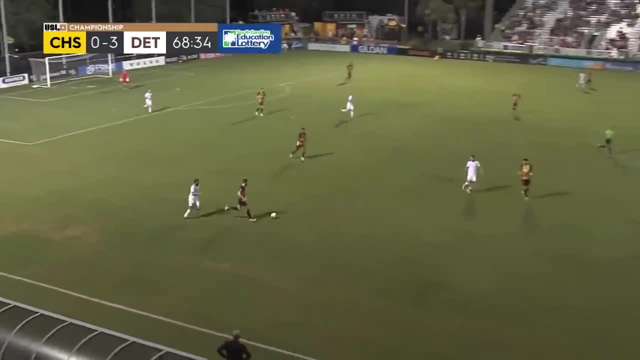 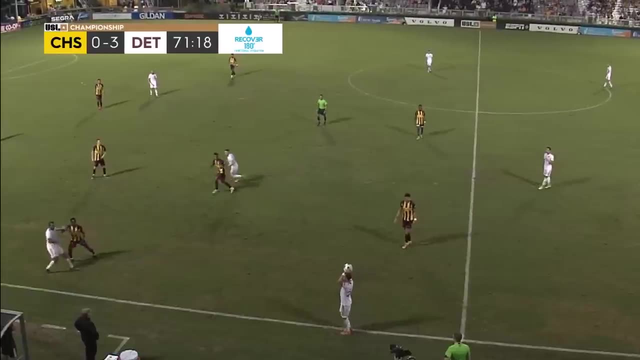 cut in front of him so that I have more time. guys to kind of try to do a long way around in order to press me, I was going to play into Andrew Booth, my center mid, so he can control the game and switch it over that far side header kind. 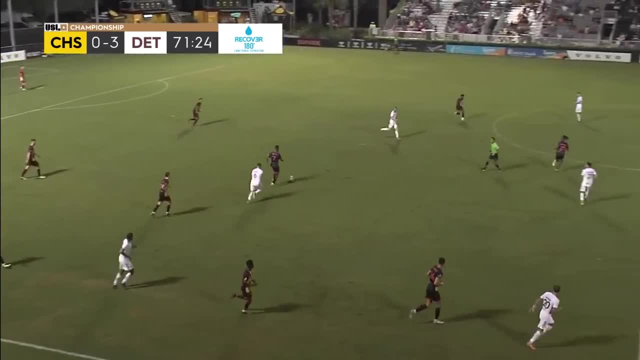 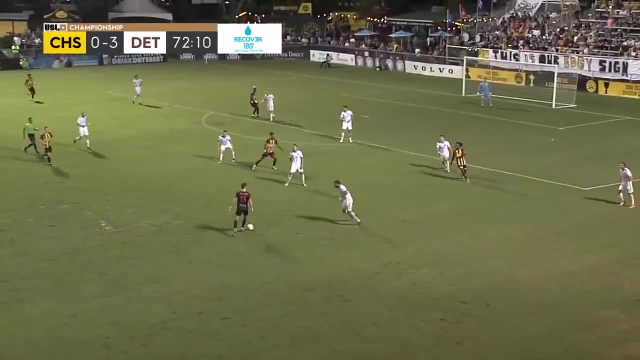 of bounces out to me and I'm just going to play the ball right into Booth. honestly, wasn't directing that header? just kind of a fast, instinctual thing. that happened quickly. and then now I'm going a little bit forward now because we need goals, so bad, so I'm receiving the ball cutting inside. I 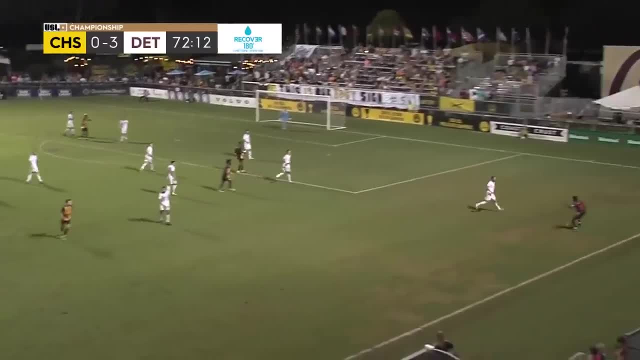 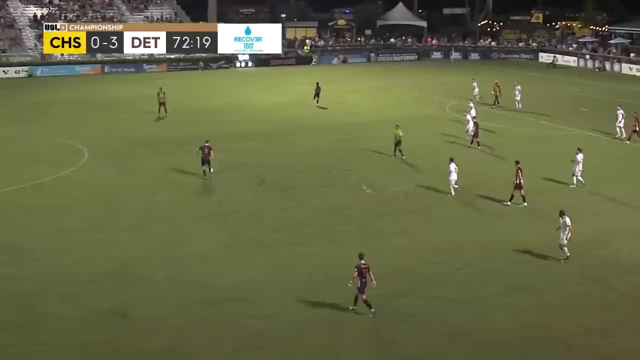 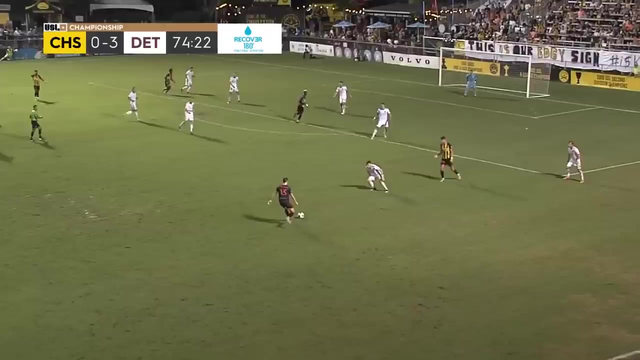 don't see what I want inside any clear passing angles. Detroit City's so compact with their lines Dexter, my, uh, my right wing back here, and this was the hard part, we just couldn't break them down here receiving the ball. I don't even look. I, just out of the corner of my eye, see a dark figure and 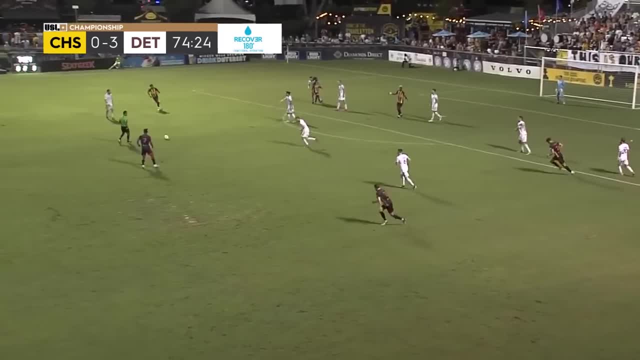 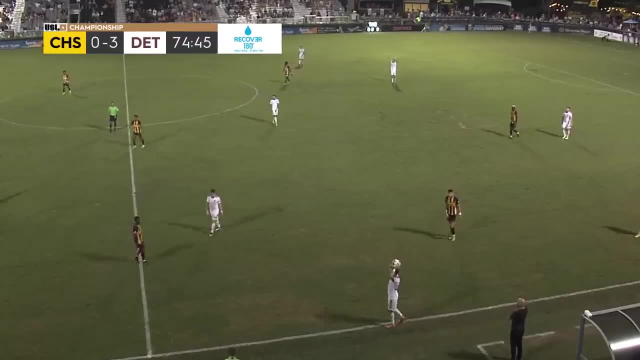 I'm looking at the ref and I end up trying to play the ref here and just goes to nobody and that's because I didn't check my shoulder beforehand and see where my players were. so because of that and easily turning over a stupid ball, winning the ball here from the throw-in and getting back in position, 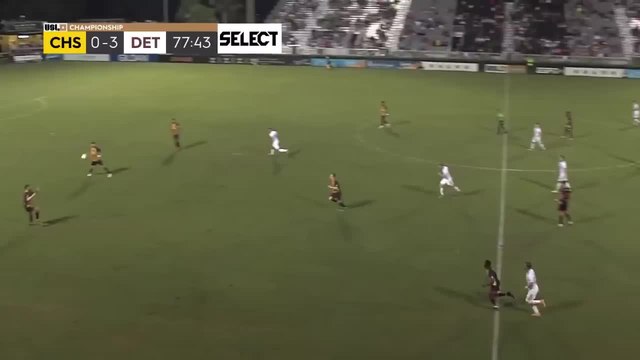 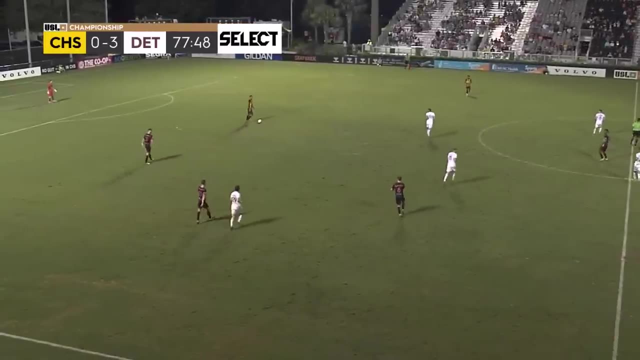 I find the ball in behind. I was about to head this into Robbie, but people are shouting: time, time, time. you know, bring the ball down, whatever. so I'm going to trust this ball down now, check my shoulder just to see where my winger's at and then play into- uh, my opposite center back over. 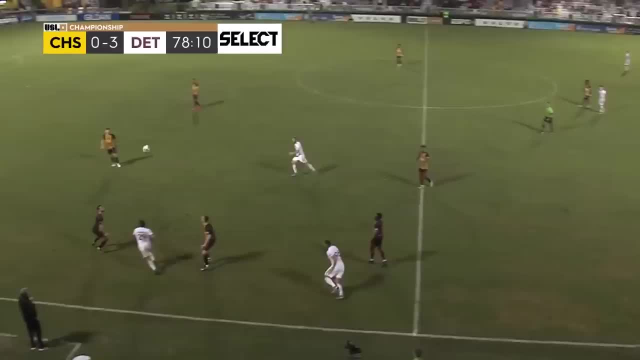 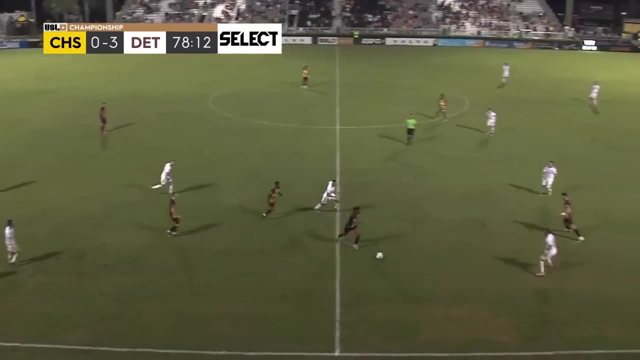 on that left side, thrown from Detroit City FC. it's going to come out to me and then immediately I'm trying to beat these three, uh, Detroit City players. try to head that ball into Booth, do a good job, to beat them and then Booth can turn and face forward. now this is a tough play. ball comes into my guy. 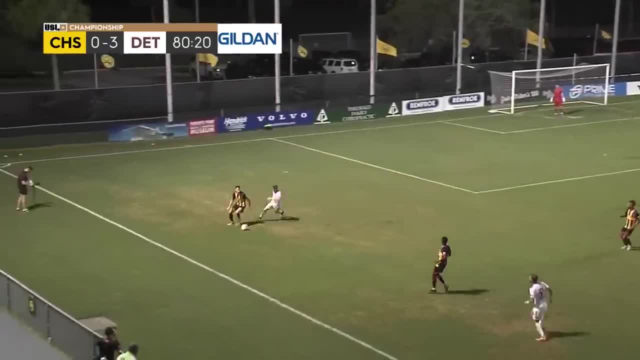 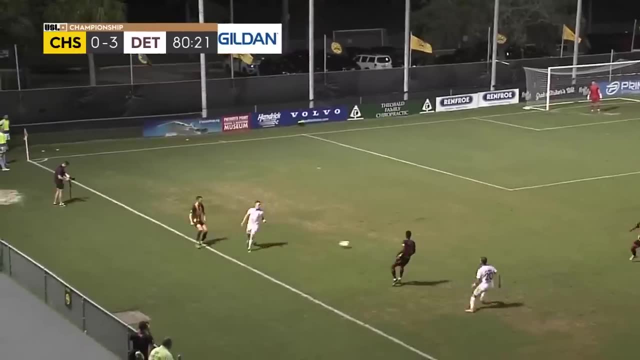 come inside and then he does a good overlapping run, but I'm still able to get there- bring this ball down and then, out of the corner of my eye, I see Booth. you see Booth is already checking his shoulder. I think this is a great decision, not just to kick the ball out. I try to play in the. 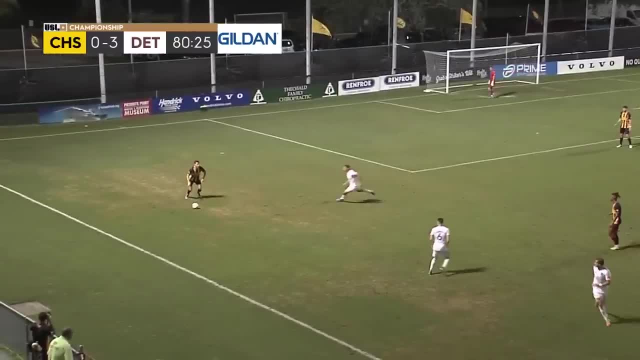 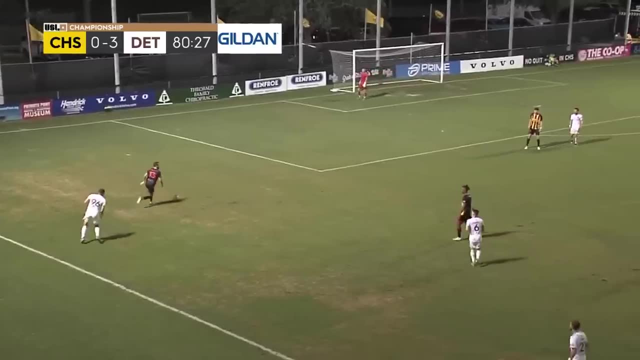 booth so we can keep. the ball ends up bouncing back to me and then this is. once again. I was looking forward and not seeing what I wanted. and this is. you have to be very careful if you're going to do a Cruyff turn just outside your box, but just with the angle of his run. I thought that. 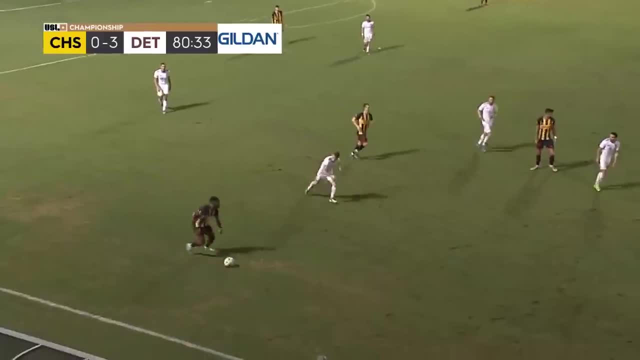 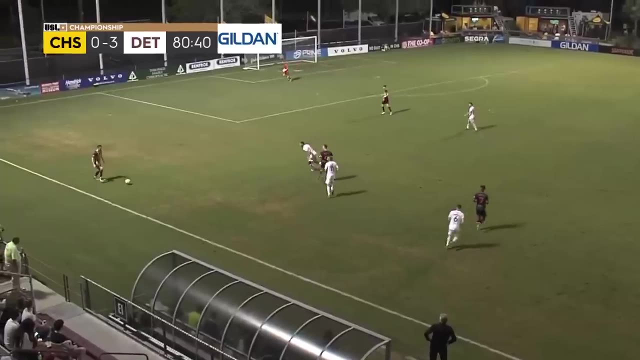 I could do it there and then playing inside into Robbie Crawford. Crawford is going to play out to Booth and I think this is fantastic ball possession and ability to break out of their, their press from us once again. ball comes back to me. looking backwards, I could play. 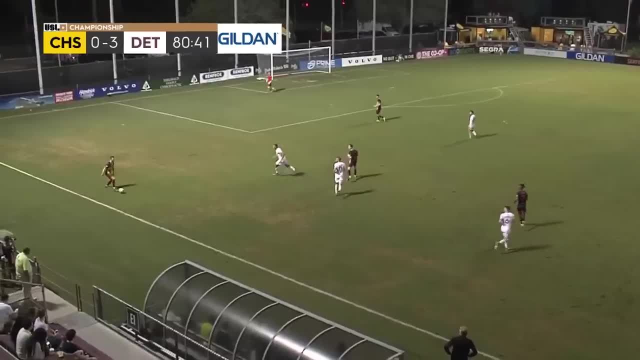 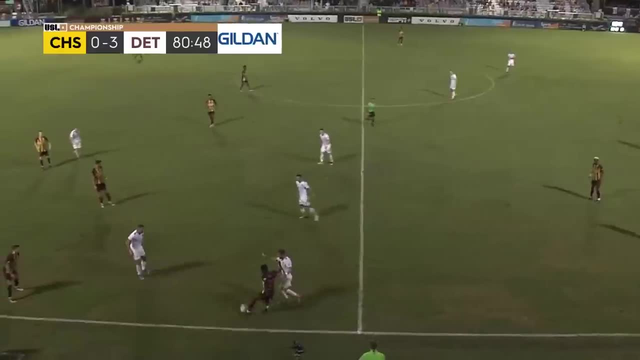 into Ugo, but I want to try to play forward and look forward. so I'm going to drive forward in front of this rounded run, uh, and then look forward into my wing back. who's going to bring this ball down into Mauro? another great passing angle here. and then Mauro finally breaks that pressure and 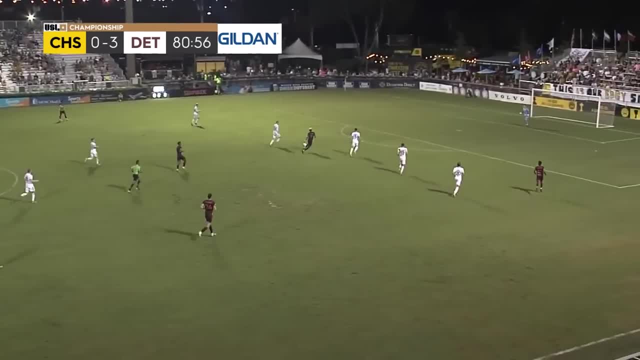 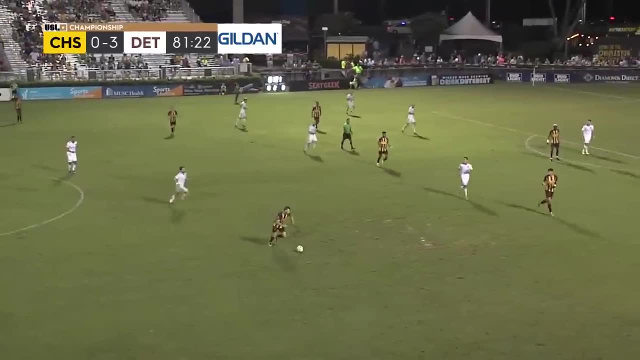 we're out. so very, very patient building from us, um, and really good that final ball wasn't there. now Crawford with the ball plays it out to me. I'm really forward in front of their line now looking forward again. look how organized Detroit City's lines are. a line. 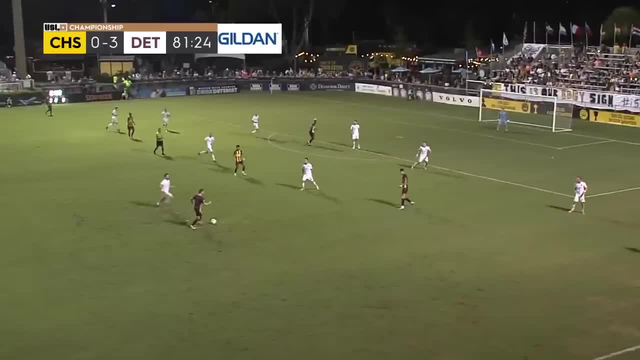 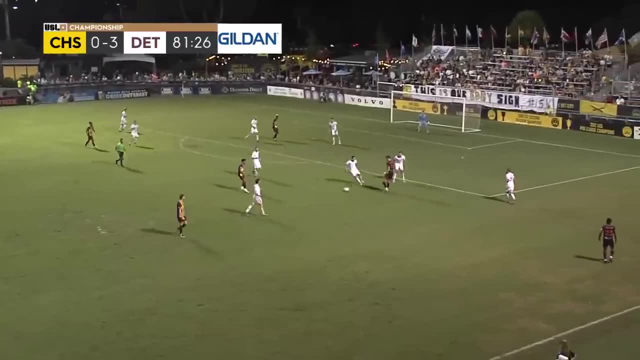 of five, a line of three and a line of one right here, and I'm just trying to find some sort of passing angle. don't see a clear one. so then I'm just going to play the simple ball tomorrow right here and we can try to build an attack just piece by piece. so anyway, Jebel has the ball, he's going. 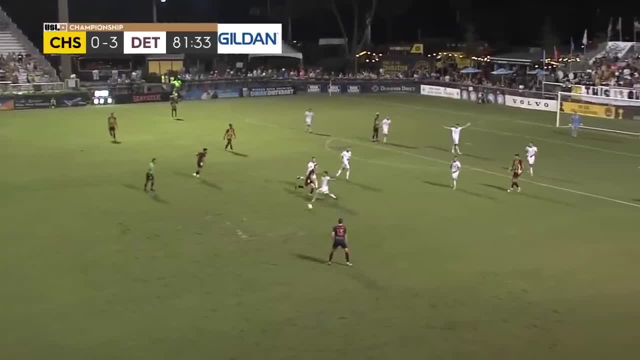 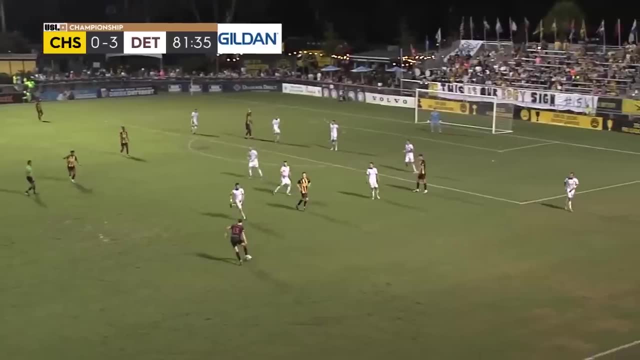 to play it back to Robbie, who's going to bring it back to this right side. I'm just in a good angle to receive this ball now and you can see the entire Detroit City players are now not in their lines. they're starting to pressure. this way, there's tons of open space on this left side, so I'm opening up. 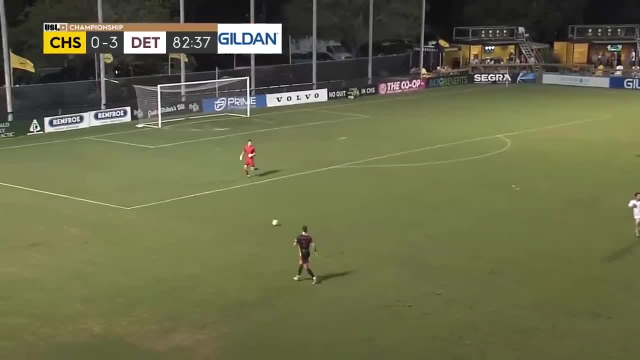 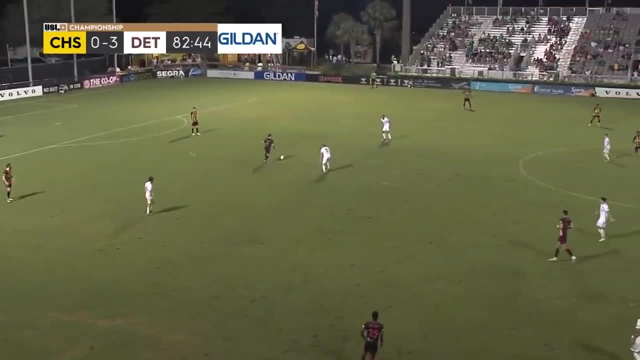 playing back. and now we're finding that left side in order to attack, receiving the ball from Ugo Ferro, my goalkeeper, just turning, and then playing into Robbie Crawford and telling him to turn, and he's going to do his his thing in the center of the field and find a great pass in the booth. we. 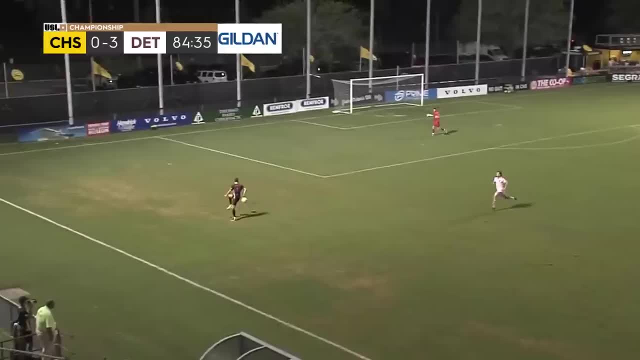 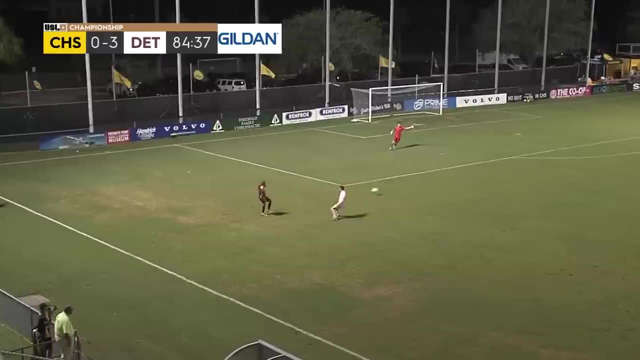 will throw once again with the ball just opening up, little tough pass, a little bit behind me just bringing this down, and in this situation this is a big trigger for the opposing team. so I'm just going to play very, very simple here, just playing across my box into my other center back, Pat, and so we can just keep the ball there instead of 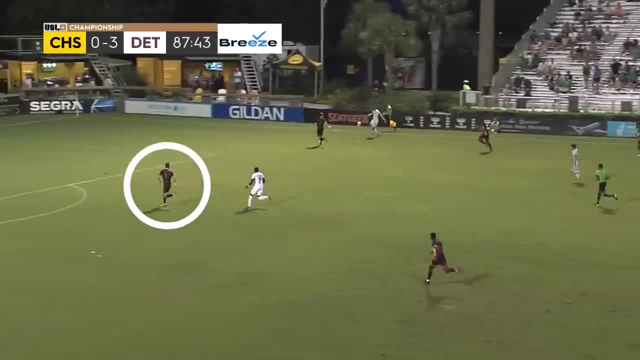 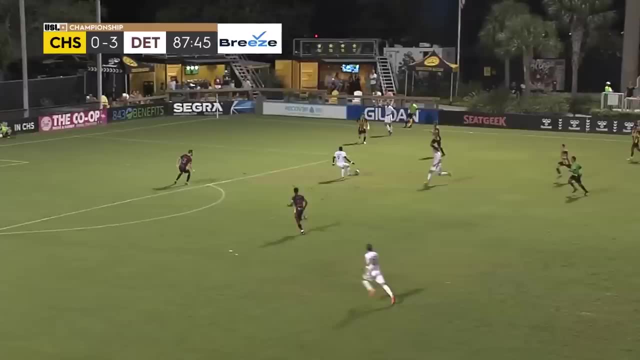 driving forward, since I don't think it's on there. a little play in behind now and then here. this is like a 3v2 situation. we've got a B on this far side. I have to be very, very careful. I'm not going to fly forward. I'm just kind of seeing what's around me, seeing my runners, and then, as soon as 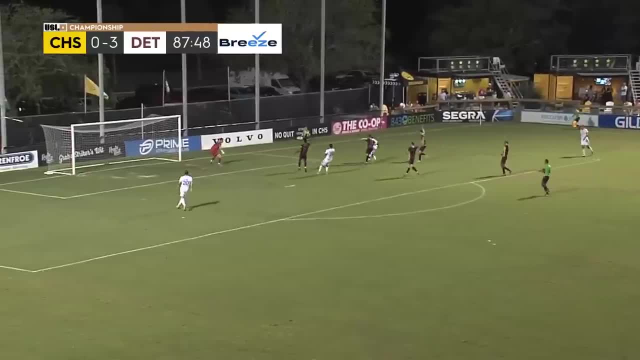 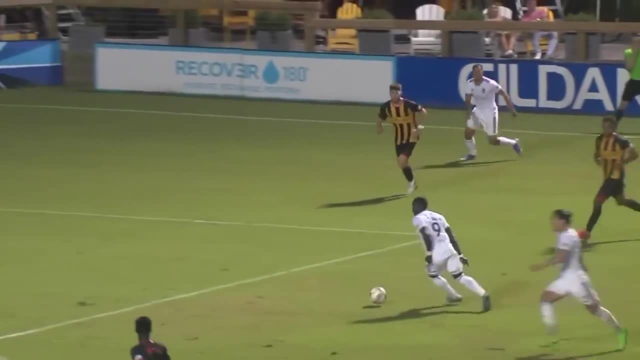 I'm able to close down the shot and just position my body in front of him. so I'm being very, very patient until he takes an aggressive touch, and then that's when I make my movement to go and attack. it's uh, it's risky though, but it's tough. in a 3v2 situation it's very, very hard to deal with. 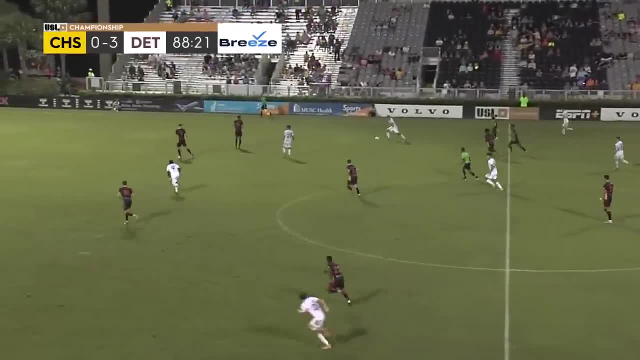 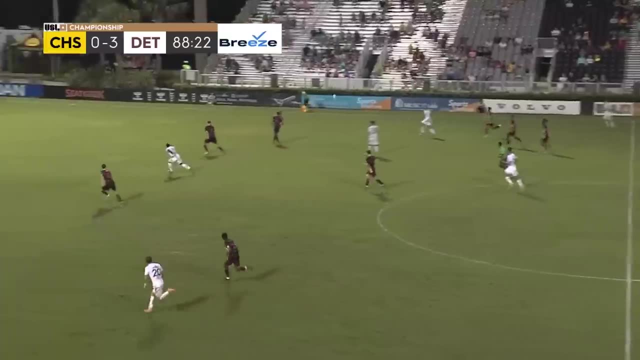 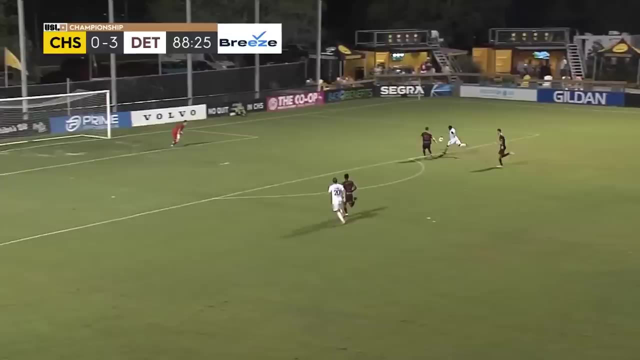 at times, but I think that was very well handled by myself, if I do say so myself. and then here I think we're too far over on the left side. I have to track it to a henna here and follow his run as a back all the way over on the left side tracking this runner. I do a good job, just to be there force. 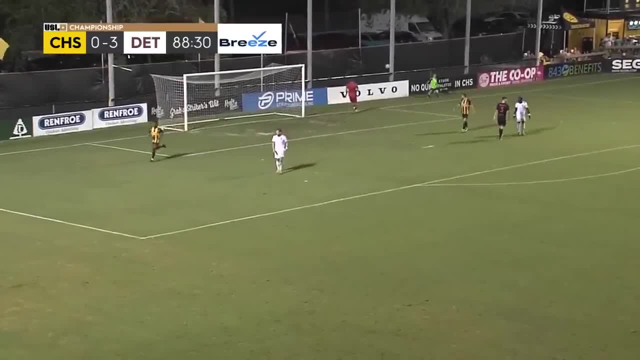 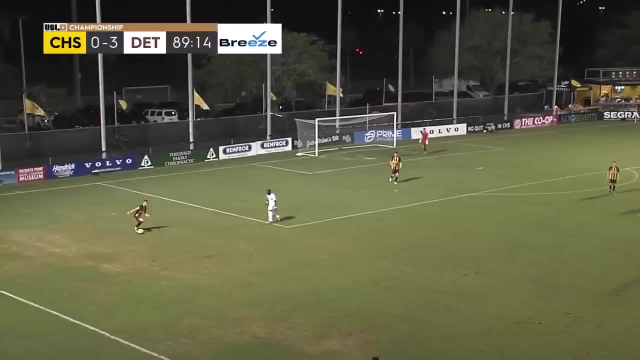 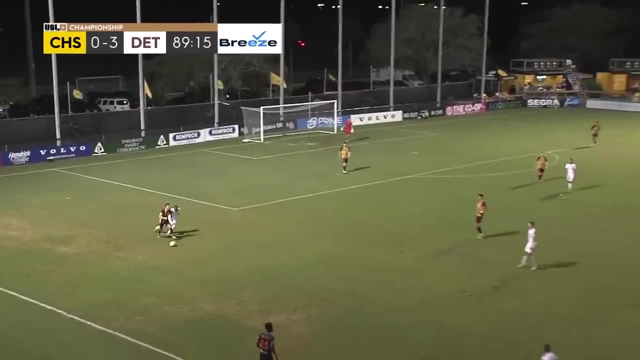 a difficult shot, still very dangerous, but if he's going to take a volley shot outside the box, that's okay. receiving the ball now. facing forward, I have some space that I want to exploit, so I'm going to drive forward in front of a two, a henna, and start to look forward here as I drive forward, not seeing. 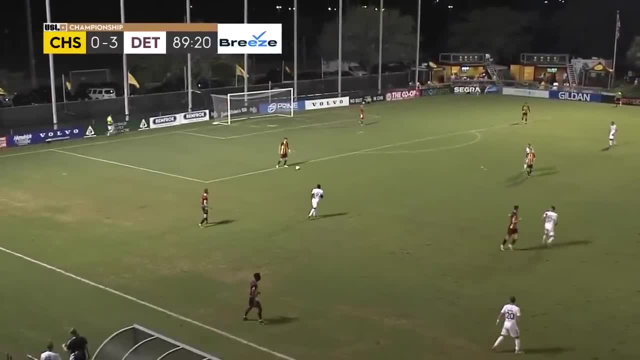 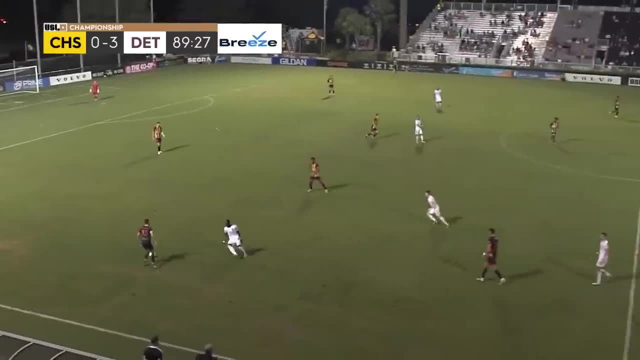 the angle that I want. so I'm going to cut the ball at the outside of my foot back into Pat Hogan. let's keep the ball once again, play in the booth. he's going to play it out to me looking forward again. I'm trying to see. I mean. 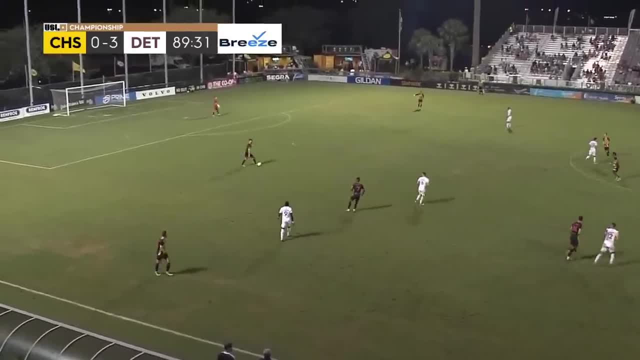 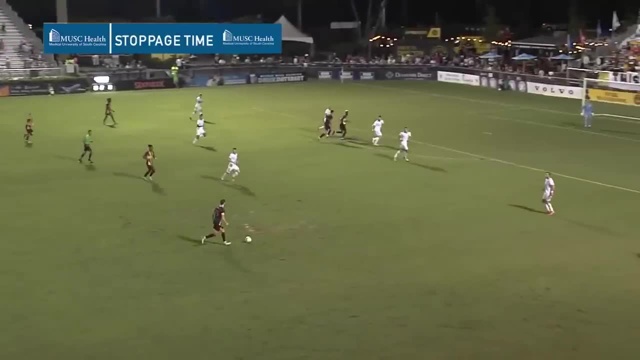 it's just tight. I mean, Detroit City's got very good positioning to make it very difficult to build there. uh, Jebel plays me out the ball. I got tons of time once again in their attacking half. I think this is a good situation to try to play this ball back post. I think I should try to aim. 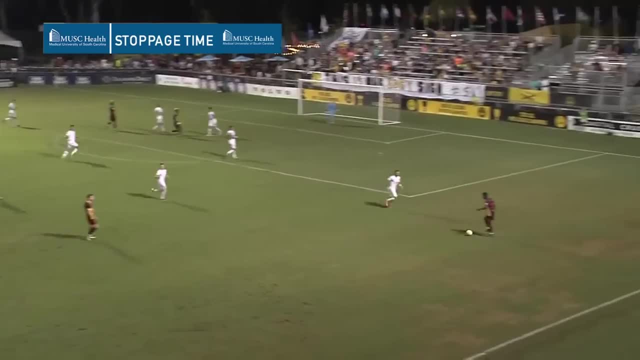 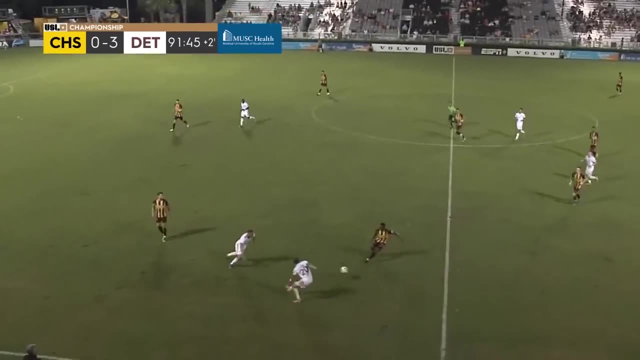 right here because we have Mauro and Augie trying to uh find that back post area but uh, Dexter does it, but now they're kind of set. I think it's still a great ball, but I think I am in a better position to cross the ball there and I think I should cross the ball there, saving the ball back from Robbie. 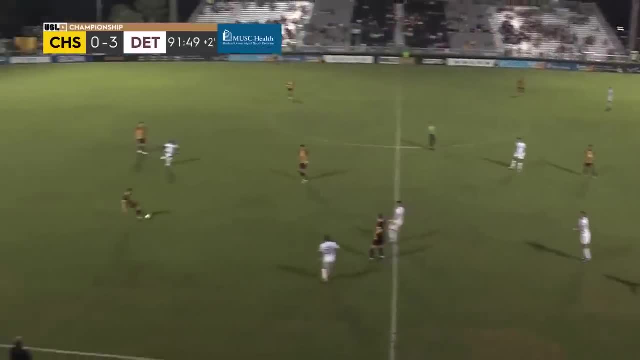 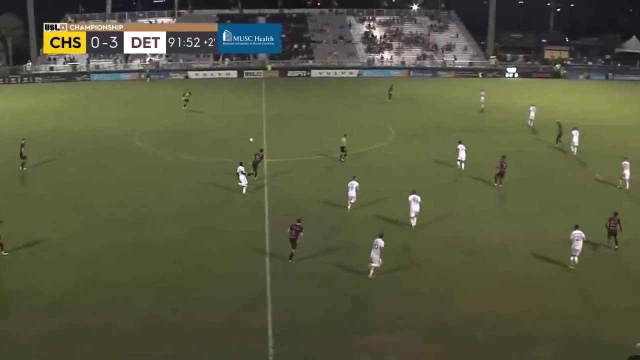 Mauro's in a great pocket of space here. so just first time, pass right into Mauro, to his left foot, so he can turn, turn and face the field, the the place that you put the ball and where you pass the ball to his left foot, to his right foot, whatever tells them if they can turn or not. 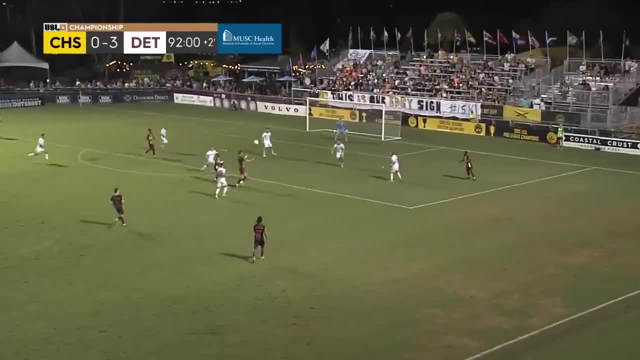 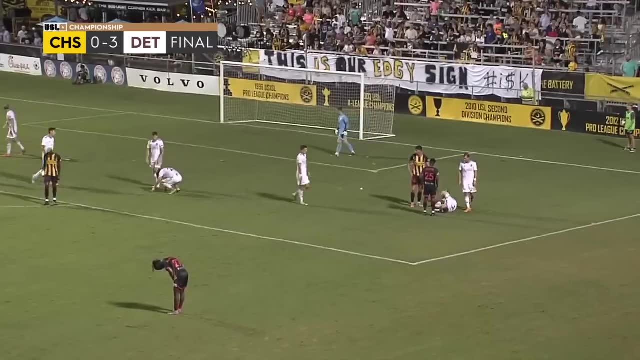 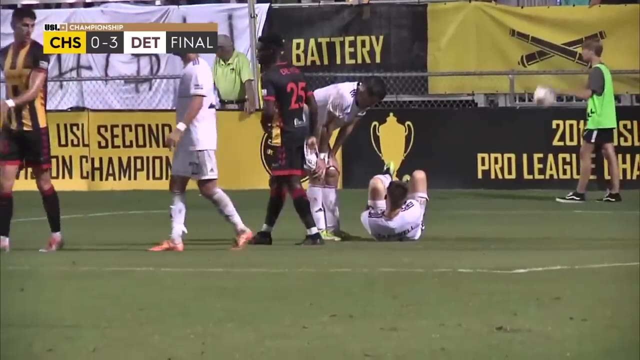 as well as your communication telling them turn or man on or whatever um. but unfortunately there's the end of the game. the referee blows his final whistle in the 93rd minute and we end up with a lead up losing three nil. so frustrating, very, very frustrating game. um little tactical positioning.